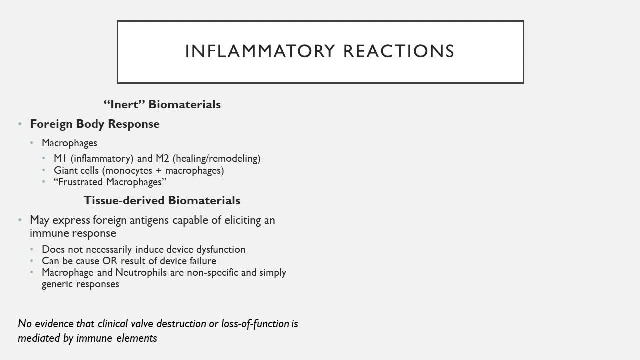 synthetic polymers, metals or ceramics or things that aren't considered natural to tissues or bodies. And then we're going to go a little bit deeper into the concept of biomaterials. We have what's described as the foreign body reaction or the foreign body response, And this 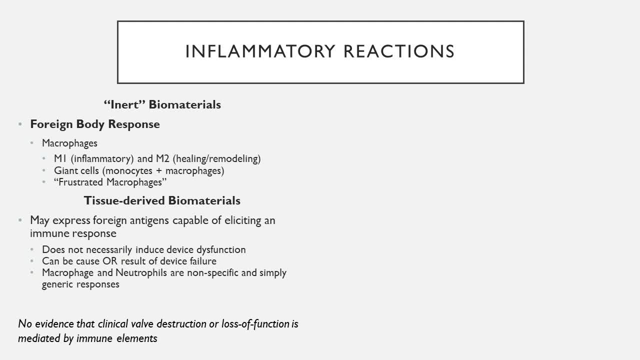 is a special form of nonspecific inflammation, meaning that there's no antigen specific to that particular material, like you would with a tissue-derived biomaterial. Now, the most prominent cell associated with the foreign body response are macrophages. Macrophages can differentiate. 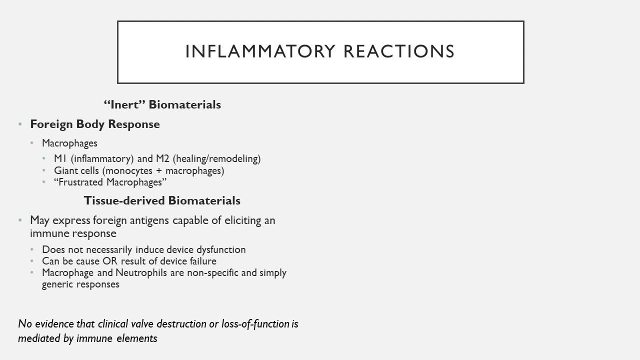 into various subtypes. The two prominent ones that I want to talk about are M1 and M2 macrophages. M1 macrophages are the ones that are most common in the body And they're the ones that are most common in the body And they're the ones that are most common in the body And they're the 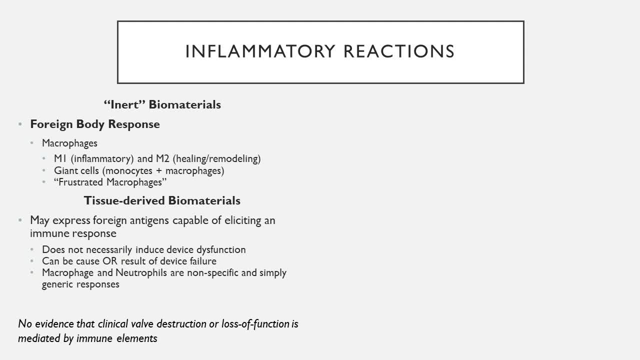 inflammatory macrophages whose primary responsibilities are to get rid of foreign bodies, whether they're pathogens, bacteria or, in our case, a synthetically derived biomaterial. They support microbicidal activity, they're pro-inflammatory and they elicit dense connective. 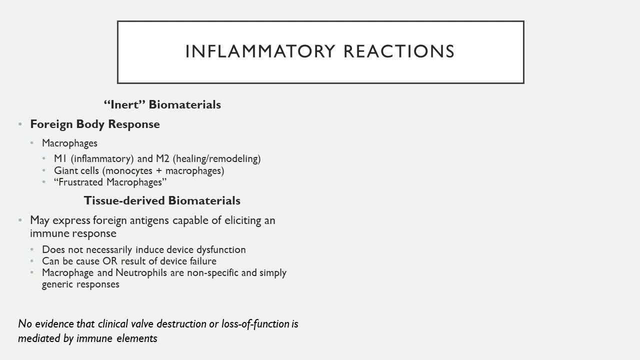 tissue and or scarring formation through fibrosis. On the other hand, M2 macrophages are not competent to eliminate pathogens And they're really just there for wound healing and remodeling. So a lot of biomaterial scientists, especially those that work with tissue scaffold and regenerative medicine, 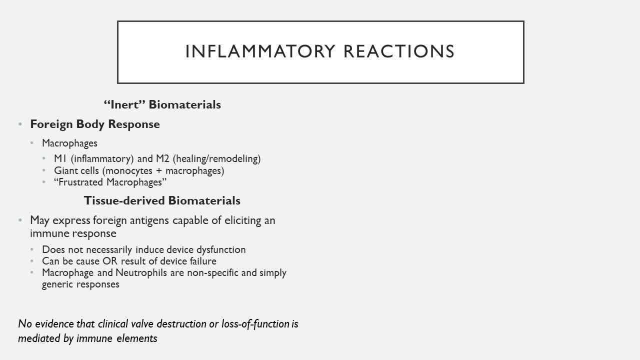 want to eventually elicit responses of M2 macrophages versus M1. Although there's also some studies that suggest that you want a sequential ordering of M1 to M2, because the inflammatory stage can help set up and support the M2 wound repair stage During particularly. 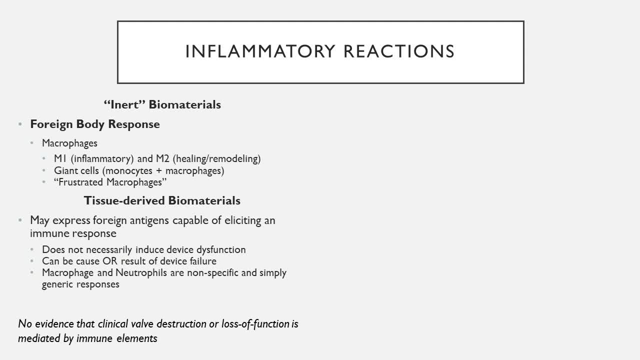 bad inflammatory reactions against biomaterials, so ones that are not very biocompatible. you might see the formation of foreign body giant cells. These are fused monocytes and macrophages that become multi-nucleated single cells that are a hallmark of a very severe inflammatory reaction. 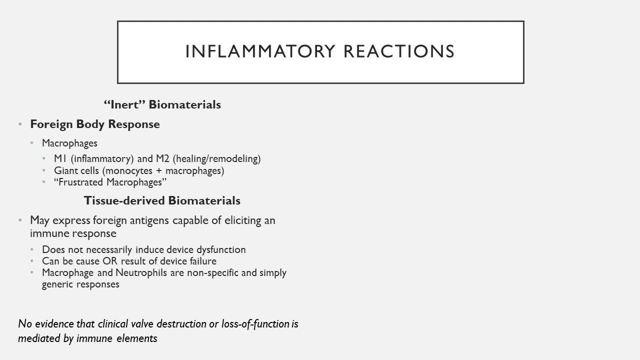 Now, lastly, I want to talk about one of my favorite terms, something called a frustrated macrophage, And I really like this term because I think it really lends a great picture of what a macrophage does. So normally a macrophage is a phagocyte, meaning that it tries to ingest pathogens by enveloping. 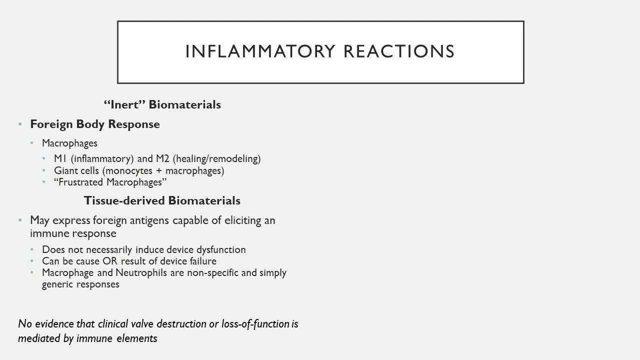 them through their cell wall and bringing them in through an endocytosis. However, when these foreign bodies reach a particular mass, like you can imagine, like a hip implant, of course a macrophage can't phagocytose it. 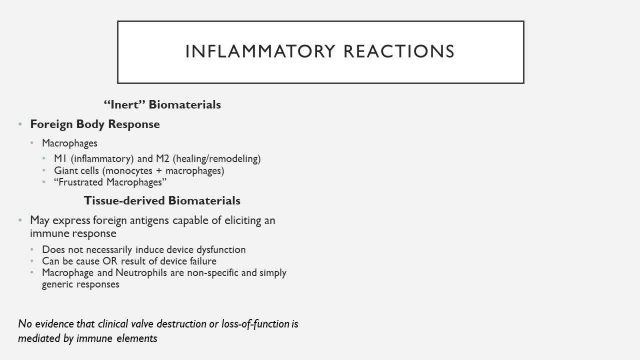 So it gets frustrated and I always picture it kind of crying because it's got to release all these enzymes through exocytosis and chemical mediators like tumor necrosis factor and interleukins that can actually cause harm to the extracellular environment. So these kind of tiers of the frustrated macrophage can in part not just deteriorate the bioplasma. 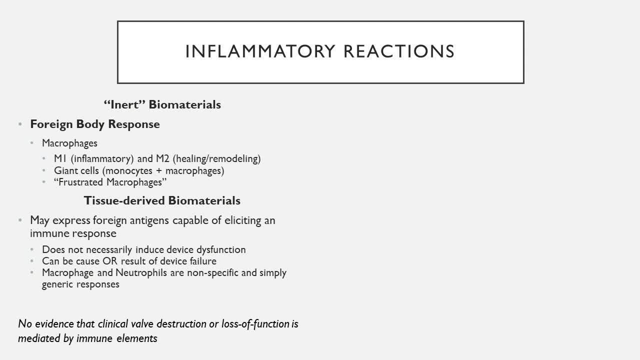 the biomaterial that we're working with, but also the surrounding tissue, and further invigorate the inflammatory process. Now, I use the word nonspecific to describe these type of reactions, because macrophages and, to a lesser extent, neutrophils don't have any specific markers for any types of materials. 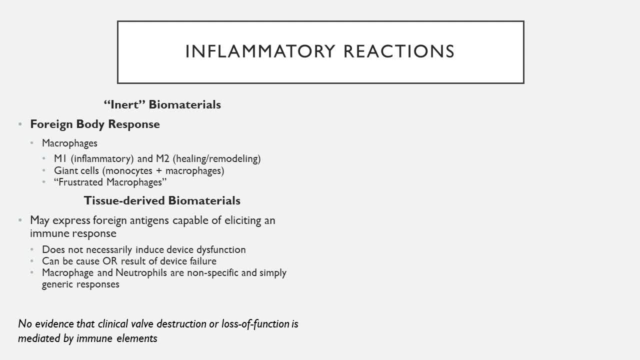 or tissues. They just have very broad recognition capabilities and that's why we call this nonspecific. In contrast, any sort of tissue derived biomaterial that we get from either different species or same species that are just genetically different will have specific markers called antigens. 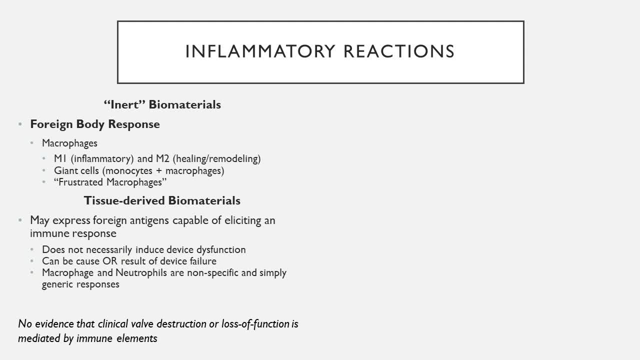 that our body has been trained to recognize even before we've been exposed to them. These are the same mechanisms through which we recognize different strains of the flu virus when given a vaccine, so that we can then learn to develop the appropriate responses against them even before we've even encountered that particular pathogen. 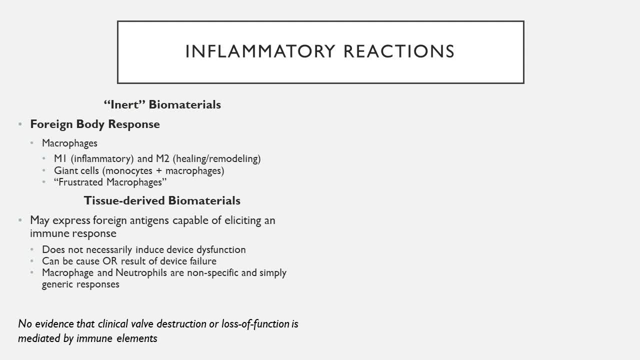 Now there are a number of different devices that use tissue derived materials, like heart valves. It's actually very common to get them from the heart. It's actually very common to get them from the heart. It's actually very common to get them from the heart. 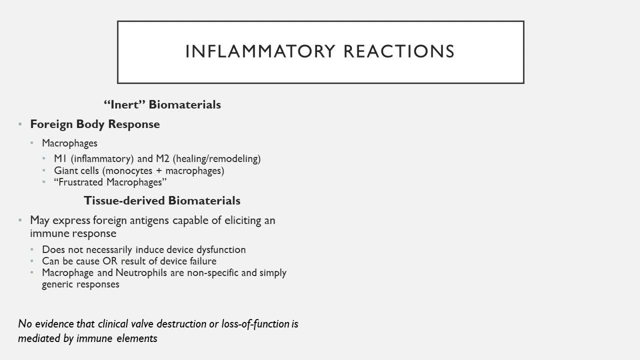 You can see that in the heart valves of pigs, tissue grafts, skin grafts and then even some scaffolding material or extracellular matrix for some kind of new generation tissue remodeling or tissue engineering applications. Now, the fact that these devices have been used successfully for years using tissue derived, 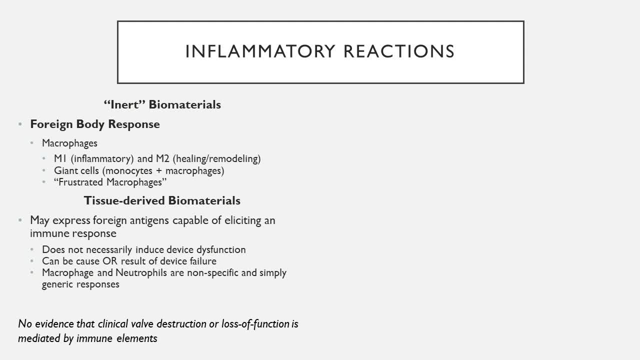 biomaterials indicates to us that just because they elicit an immune reaction does not necessarily mean that that causes some sort of device dysfunction. And lastly, in the case of heart valves there's been no clinical evidence by any means that clinical evidence where the valve destruction or loss of function has been mediated or linked to. 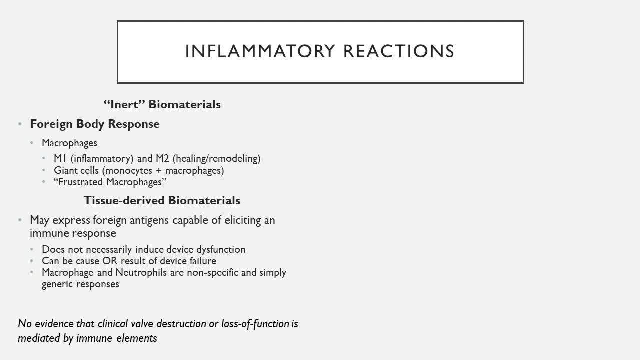 immune elements. so again, i just want to stress that just because you have an immune response to a particular biomaterial or device doesn't mean that that's going to lead to the device failure. now, in order to determine that if a failure of a device is linked to an immunological reaction, 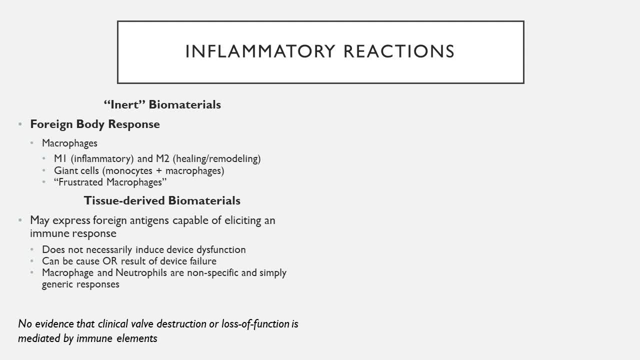 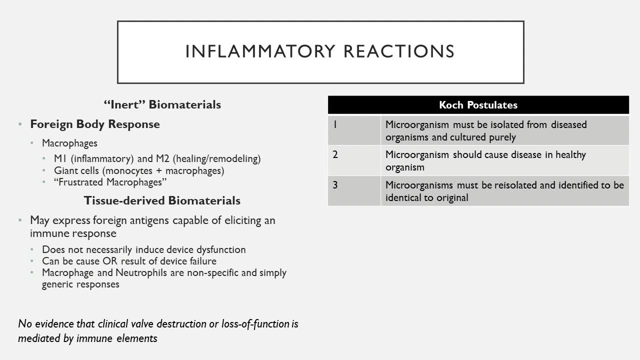 biomaterial, scientists have adapted postulates developed by german physician robert koch that were originally used to define if an infectious agent was responsible for a particular disease. originally. if an infectious agent was thought to be linked to a particular disease, scientists would take that agent from a disease host, inoculate it in a particular animal and see if. 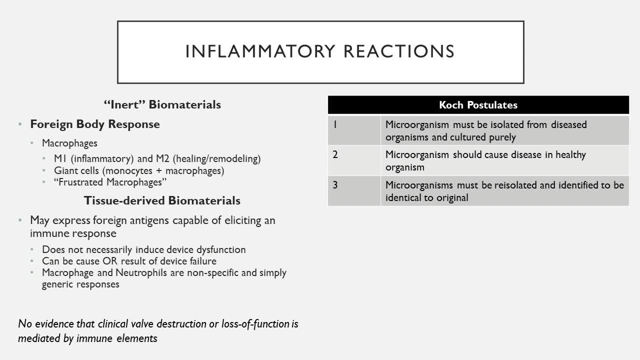 that also caused lesions. and then, lastly, they would recover the particular agents within those lesions to see if it was that same agent from the original diseased host. now, the way biomaterial scientists have adapted these postulates is by using the same agent from the original disease host and 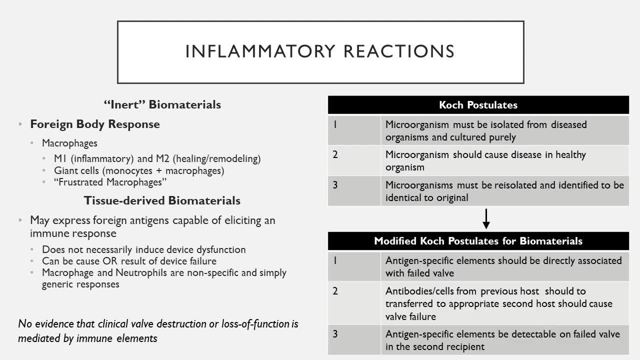 mirror these exact same three postulates. First, scientists would first determine if an engine specific element, like antibodies or cells, are somehow directly associated with, for instance, a failing valve. Second, these antibodies or cells from the first experimental animal should then be transferred to a second animal with that same particular device. Then, by transferring those, 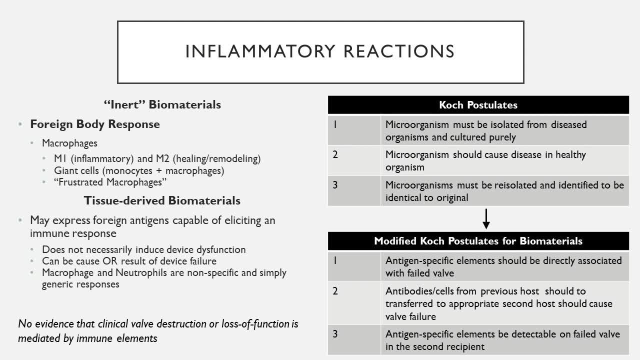 antibodies or cells, that second animal should also have a failed device. Lastly, those adoptive transferred cells or antibodies should be detectable on the failed device in the second recipient. If these postulates hold true, then scientists could then determine and conclude that immune responses were responsible for the failure of the device. 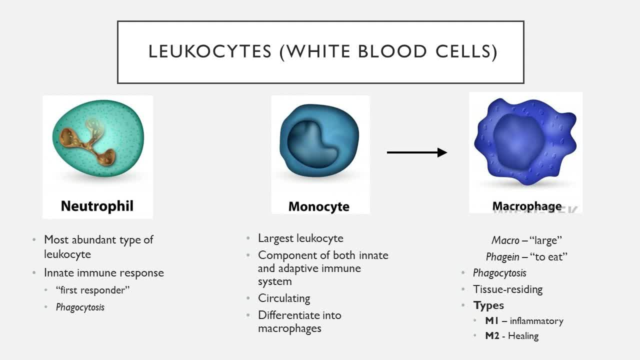 Now I realize I mentioned these blood cells both earlier in this lecture and also in previous lectures, but I wanted to give a brief overview of the different types of leukocytes, which is just an umbrella term for white blood cells, which differentiates them from red blood cells. 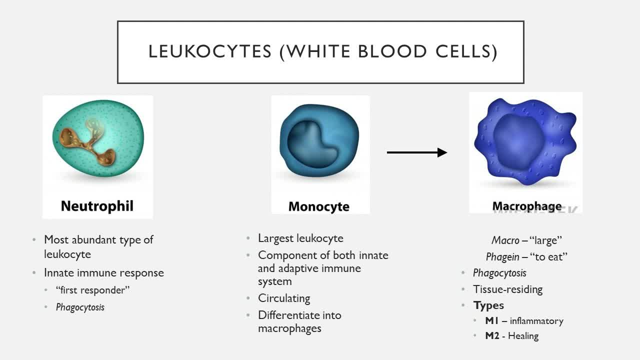 and platelets. Now, the most abundant type of leukocyte is a neutrophil. Neutrophils are often called polymorphonucleic cells because their nucleus is this multi-lobed sort of structure, like you see on the picture. During an inflammatory response, neutrophils are often called the first. 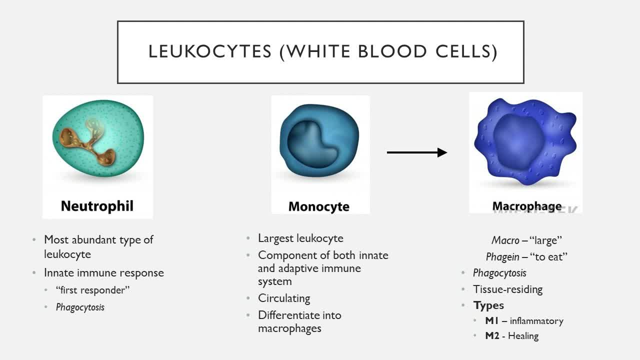 responders because they're first of all abundant in higher concentrations. They respond faster to chemokines, which are a type of messenger proteins that give migration signaling to cells, And they're also a type of phagocyte. so that means that 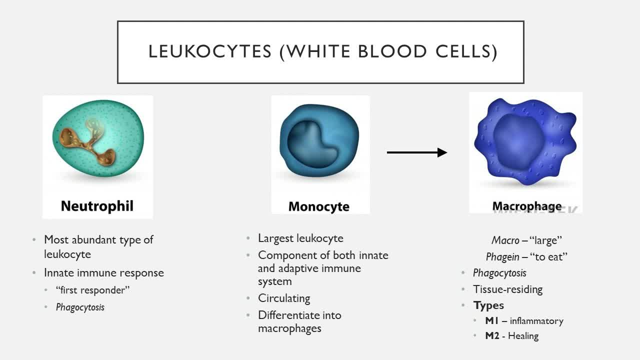 part of their job is to ingest pathogens, especially during the early stages of infection. I also mentioned the term monocytes, which are the largest type of leukocytes and they're primarily found in circulation And they have components of both the innate immune reactions. 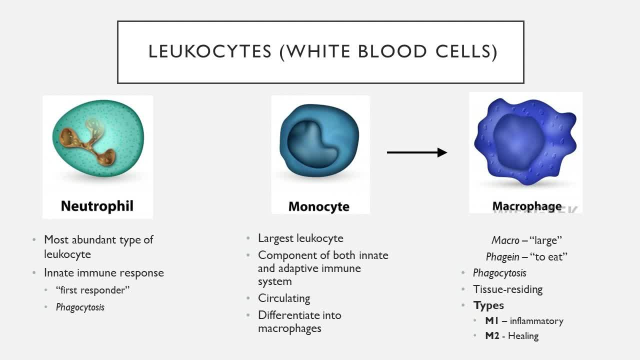 and adaptive immune responses, because they do interact with T cells during later stage. adaptive immune responses: They're circulating to contrast them into their neutrophils, which are the most abundant type of leukocytes, And they're also a type of phagocyte. 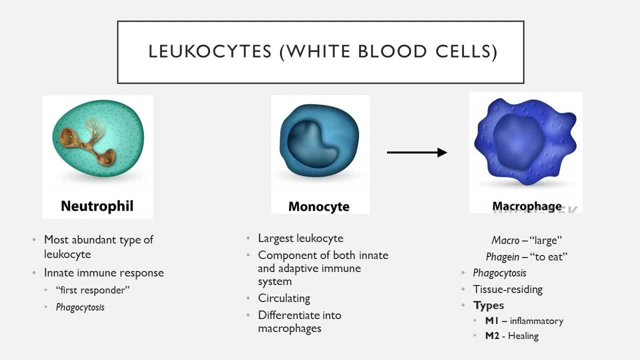 which is the most abundant type of leukocytes, And they're also a type of phagocyte, which is the most abundant type of leukocytes, And they're also a type of phagocyte differentiated effector forms, which are called macrophages. Now, monocytes typically turn into macrophages. 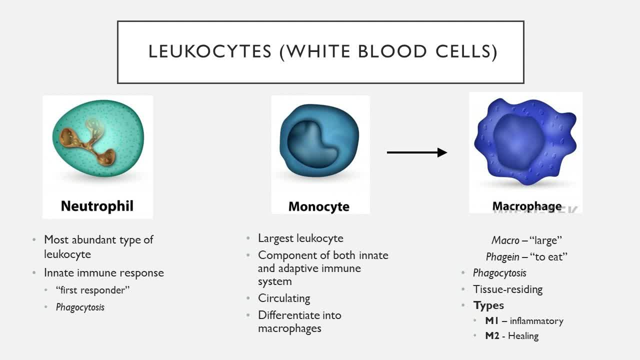 at the site of inflammation, which is usually in the tissue. So I usually think of monocytes being in circulation, macrophages being tissue. Now, the name macrophages is derived from two Greek words, being macro, which is large, and then phagium, which means to eat. So even the name implies that. 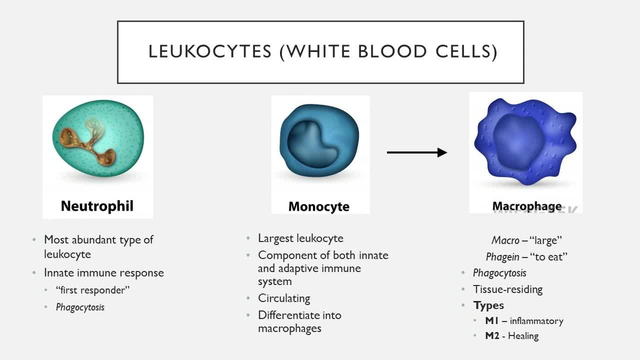 they're a type of phagocyte, meaning that they undergo phagocytosis, They ingest cells in part by pinching off their lipid bilayer cell membrane to then go into the cell membrane, And then they're then taken- particulates or pathogens- through these endocytotic vehicles, As I mentioned before. 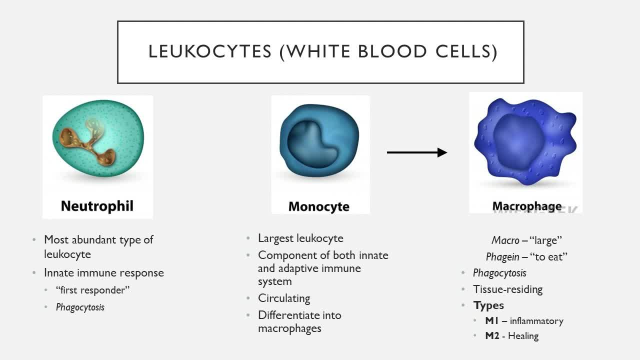 there's two major subtypes that we'll be referring to. There's the M1 subtype, which is the pro-inflammatory cell, whose job is to get rid of phagocytose cells, And then there's the M2 macrophage, which really has no inflammatory or phagocytic actions and is primarily responsible. 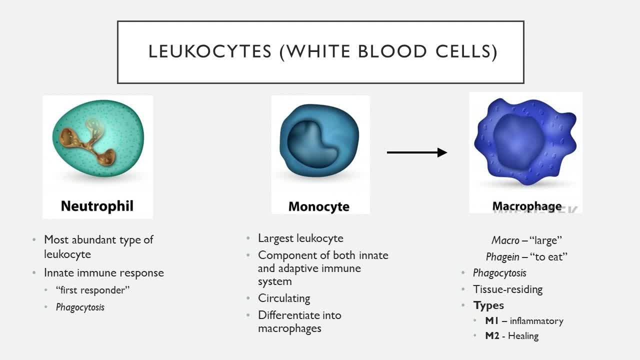 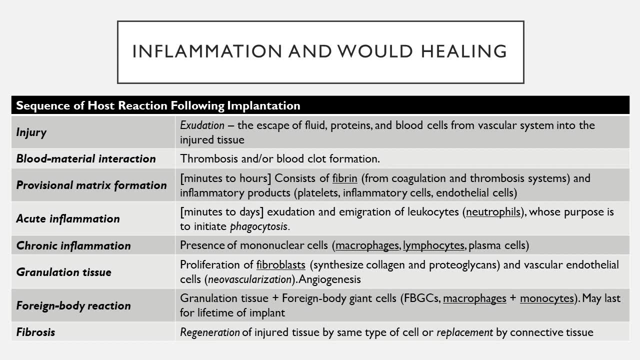 for wound healing and tissue repair. Now that serves as a nice segue into the sequential steps that are involved in inflammation and wound healing. Now inflammation in general just serves to contain, neutralize, then dilute and then finally wall off whatever injurious agent or 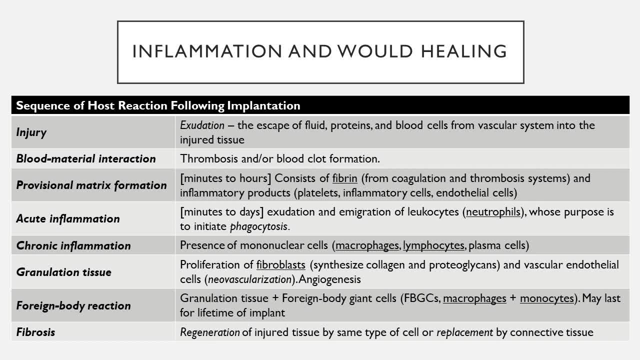 process has happened to that particular tissue And then, after that, comes the wound healing to repair that certain process. Now, the very first step in this process is obviously the actual injury, which is followed by this process called exudation, which is the escape of fluid. 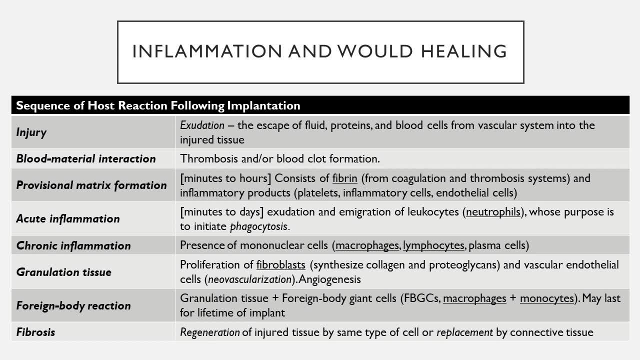 proteins and blood cells from the vascular system into the site of injury. Now, as blood brushes into the site of injury, this sets off a number of different blood material interactions where thrombus and blood clot formation occurs. Now, the purpose of this is: 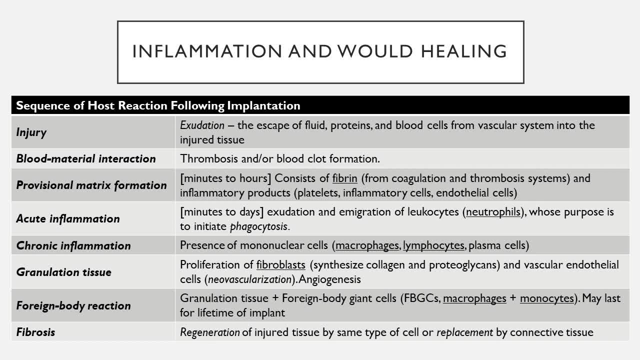 really to block off other vascularized areas so that further bleeding stops. So this just kind of acts as a plug. A lot of these same processes occur during the next step, which is the provisional matrix formation, which consists of both fibrin and inflammatory products like platelets. 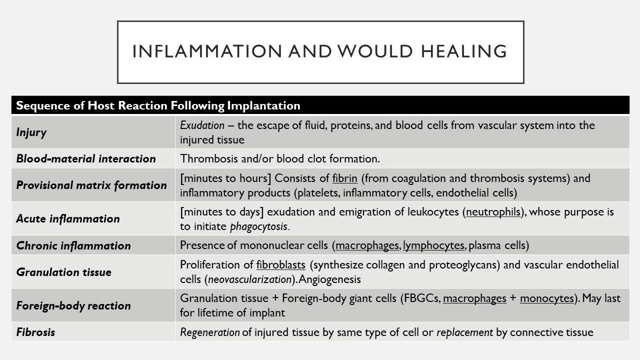 inflammatory cells and endothelial cells. Now, as blood brushes into the site of injury, this sets off a number of different blood material interactions where thrombus and blood cells occur. Now this matrix formation serves a few purposes, but basically it's a hosting site that allows for cell migration for both inflammation. 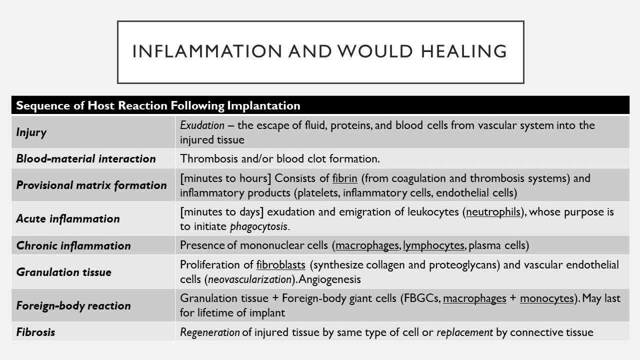 and then also revascularization during the wound repair process. Now, as we learned in our previous lecture, inflammation can occur in two sequential steps, the first being acute, which occurs over the order of minutes to days, And this is marked by the presence of leukocytes, primarily by 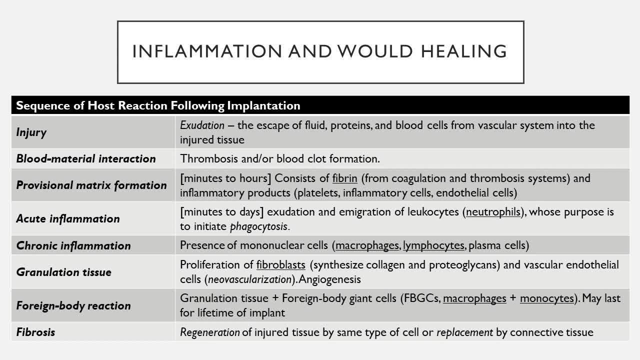 neutrophils. So I want us to associate neutrophils with acute inflammation Now, as bacteria and pathogens enter the site due to the original injury. now, the job of neutrophils is not to completely kill off all of these pathogens that have just entered, in part because they're just 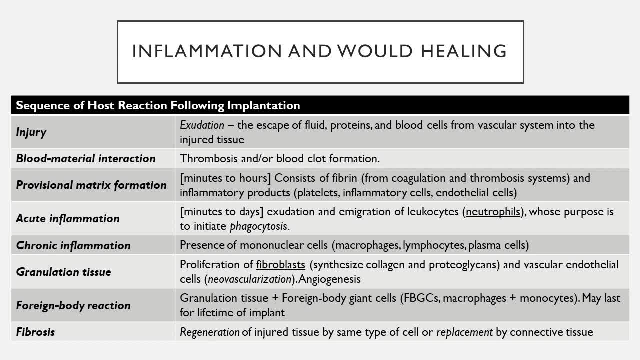 not able to. they don't have the capacity or the strength for it, And really they're meant to stave off a rapid spread of these pathogens and wait until all the mediators of chronic inflammation and more sophisticated components of the adaptive immune response can potentially take over. So 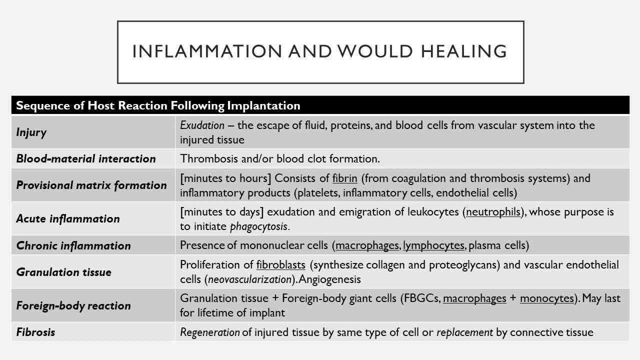 that brings us to chronic inflammation, which we see the presence of mononuclear cells. Remember again that neutrophils have these multi-lobed nuclei. This is in contrast to macrophages, which I want us to associate with. 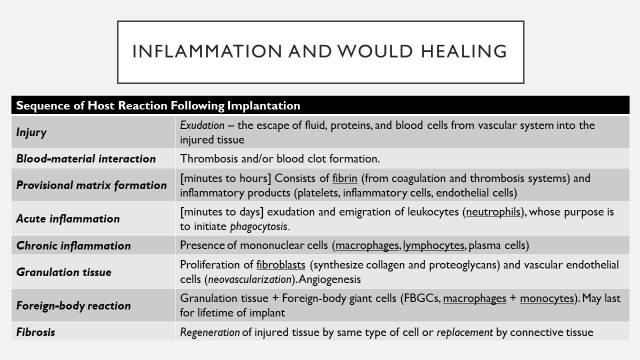 chronic inflammation, particularly with inert biomaterials. Then there's also lymphocytes which react specifically to tissue-derived biomaterials and then also other plasma cells. Now we're sort of entering the wound healing and repair process, because now we have the formation 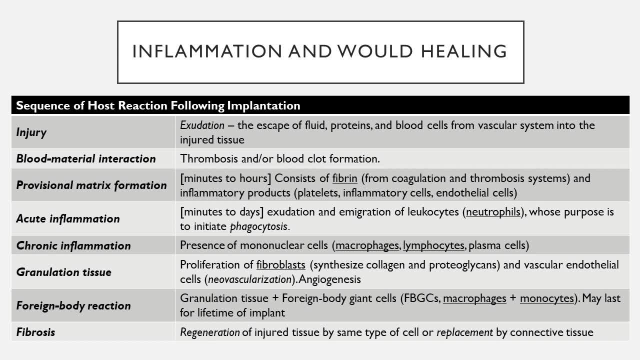 of granulation tissue, which is seen by the proliferation of fibroblasts, which are used to synthesize collagen and proteoglycans, and other vascular endothelial cells that are involved in angiogenesis, which is just the rebuilding of blood vessels. The name of this tissue is actually derived from the fact that 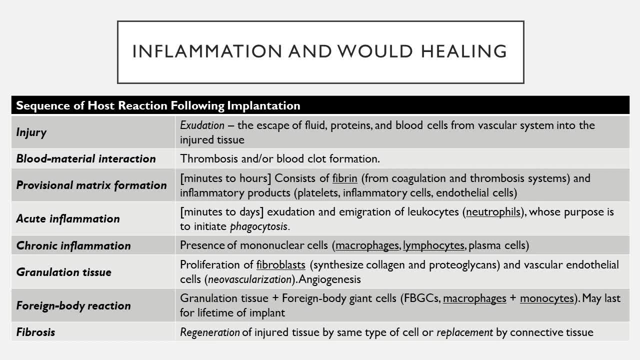 it has this really pink and soft granular appearance. So I'll show you a picture of that in the next slide once we get to it. Next up, the foreign body reaction is really a continuation of the granulation tissue formation with the combined presence of macrophages and then to a greater extreme amount, as we discussed before. 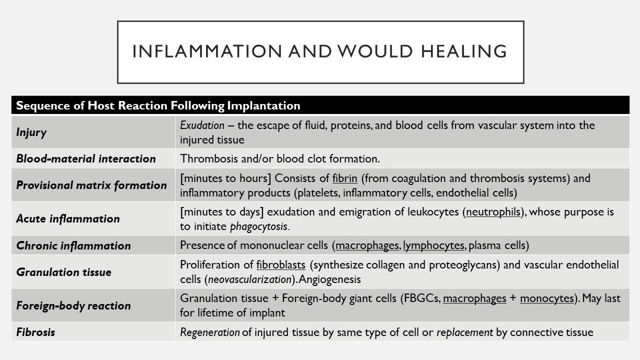 foreign body giant cells, which are sort of fused macrophages and monocytes that create this multinucleated singular cell. that's the combination of those two. Now I want to point out that all foreign bodies undergo this type of reaction, so it's not necessarily a bad thing to have this. 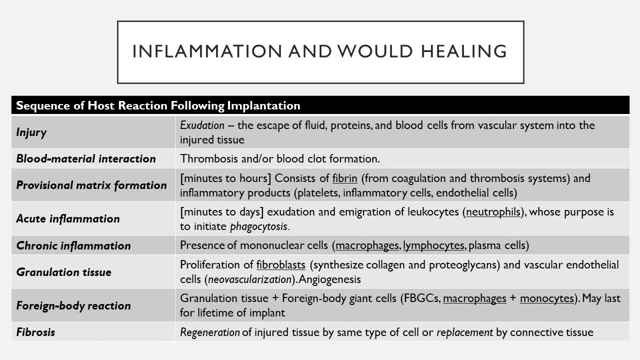 occur. In fact, we can gauge the biocompatibility of a device in part by the thickness and appearance of the foreign body reaction or the foreign body tissue formation around it. In fact, if we see a relatively flat and smooth surface around a material with just a thin granular tissue with 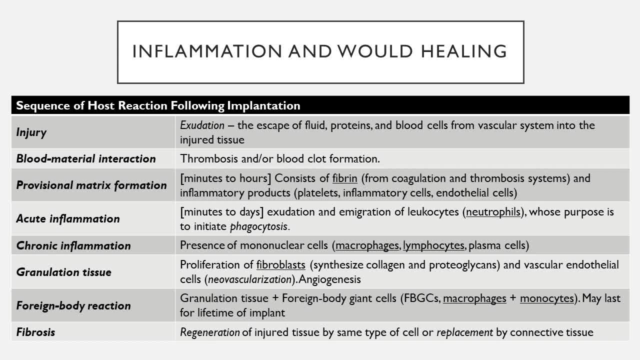 macrophages that are only one to two cells in thickness, then we know we have a highly biocompatible implant. If we see ones that are much thicker, have a lot more macrophages and also the presence of the foreign body giant cells, then we know we have a poorly biocompatible implant. 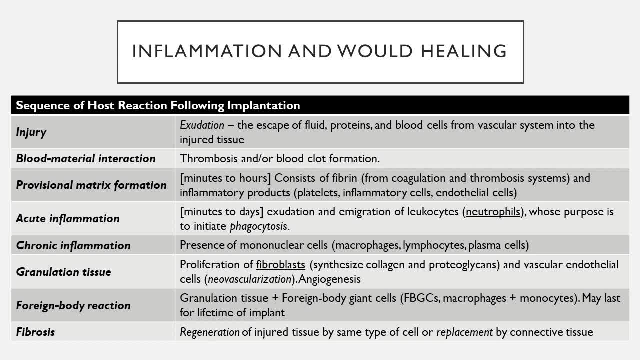 So we want to make sure that we have a really healthy response to any type of biomaterial and any device that goes in the body typically is going to see this over the lifetime of the implant. Now the last step into this long injury process is the actual repair process. Now what? 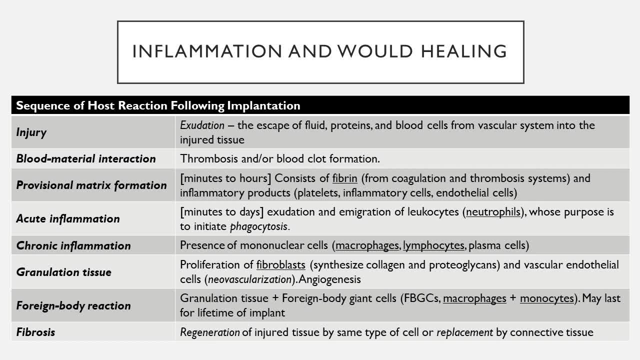 biomaterial scientists really want to strive for in the ideal scenario is a complete regeneration of the injured tissue by the same type of cell. What always happens to some degree is a process called fibrosis, which is a replacement of the injured type of tissue with a new type of tissue. 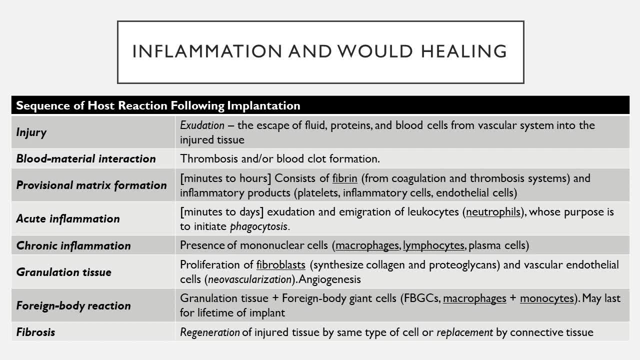 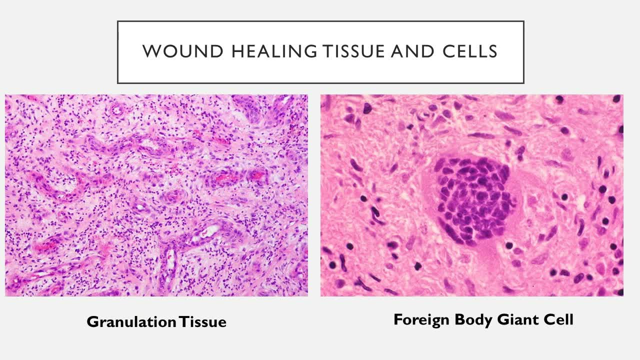 and this is really what scar formation is Now, in these two pictures we have great histology samples of the wound repair and inflammatory process. On the left we have an example of granulation tissue. You can even see why it gets its name. It looks granular in appearance. 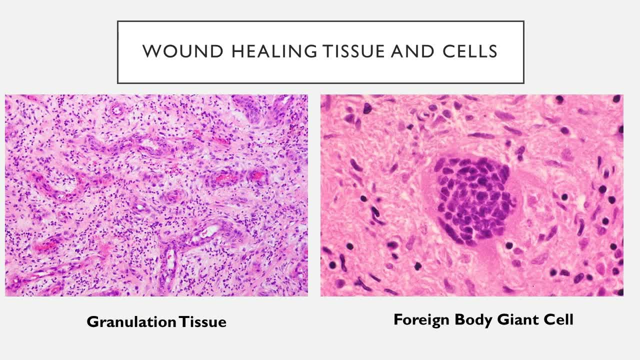 in part because of the staining of the three types of cells that are prominent during this process. There's always macrophages, and the extent of which is dependent on the inflammatory response, and then we have non-immune and non-inflammatory cells, like endothelial cells, which are 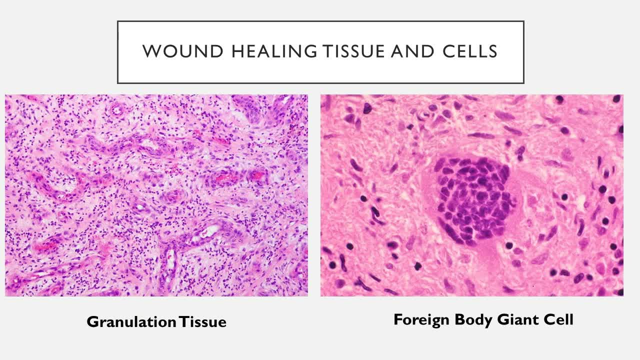 necessary for the formation of new blood vessels and then fibroblasts that synthesize collagen and proteoglycans. On the right-hand side, we see an example of what you don't want to see, which is that of a foreign body giant cell, which is a mixture of monocytes and macrophages during 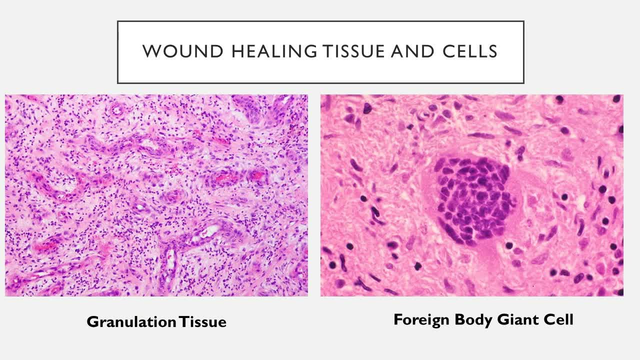 prolonged inflammatory states that, in an attempt to phagocytose or eat whatever biomaterial that is way too large for them, they actually fuse together. So this is a single multi-nucleated cell made of single monocytes and macrophages that have combined together. Again, the theory is that they 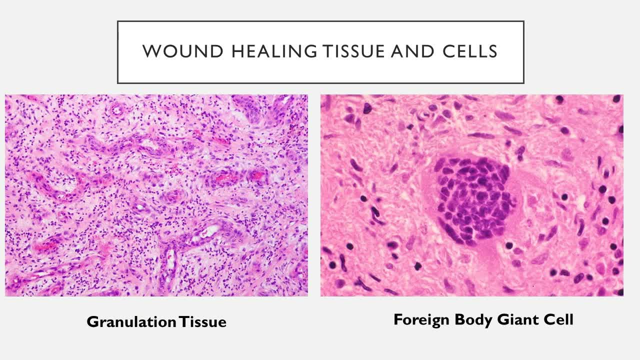 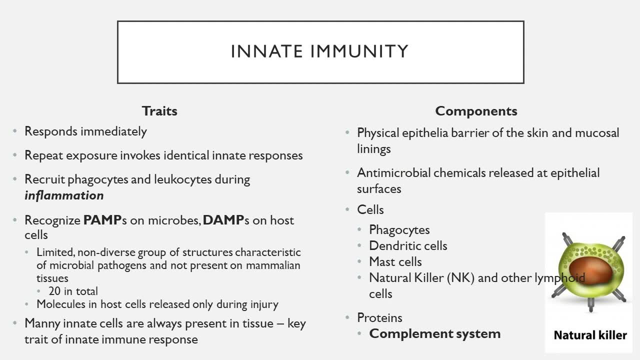 want to eventually grow so big that they can envelope whatever biomaterial they're up against. Now. what dictates the path of inflammation and how rapid or strong of a response it is is the immune system, and there's two branches of the immune system. There's innate immunity. 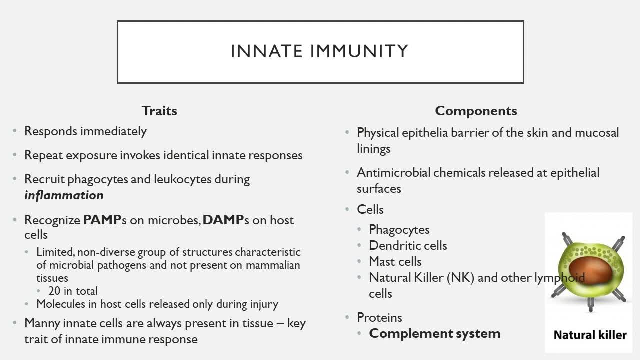 and adaptive immunity Now innate immunity gets its name because we're sort of born with it and it's built into our immune system from the start. It doesn't have to adapt, just like adaptive immunity has to In part. it responds immediately. 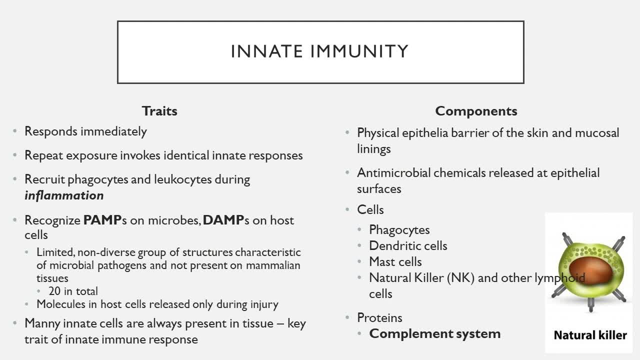 so it's always the first line of defense, and then adaptive immunity always takes over after some time. Repeat exposures always invoke identical innate immune responses. It can't learn and adapt for specific responses. It doesn't have memory. These all stand in contrast to adaptive. 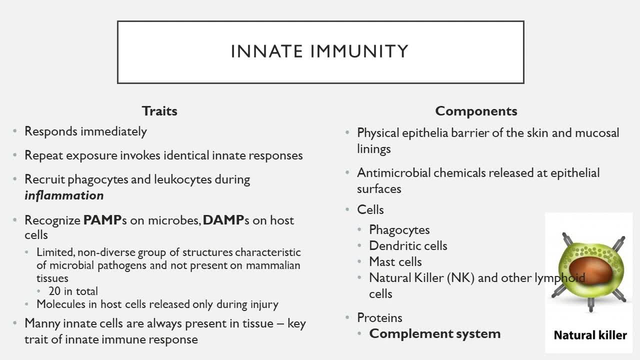 immunity, which can respond different ways in secondary and tertiary attacks. The key fighting mechanism for innate immunity is inflammation, where it recruits phagocytes, another leukocytes, during this process, usually at the site of infection or inside of wound repair and healing. Now, what triggers these responses are the activation of pattern recognition receptors. 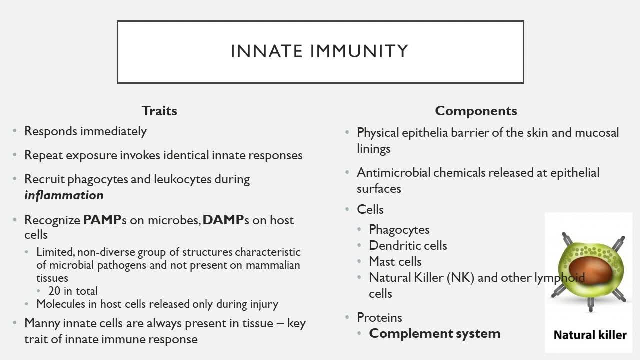 on these cells to two different categories of molecules. One is pathogen-associated molecular patterns, that's PAMPs, which are found on microbes and other foreign objects, and then damage-associated molecular patterns, which are found in our own host cells. So the PAMPs, the pathogen-associated molecular patterns, 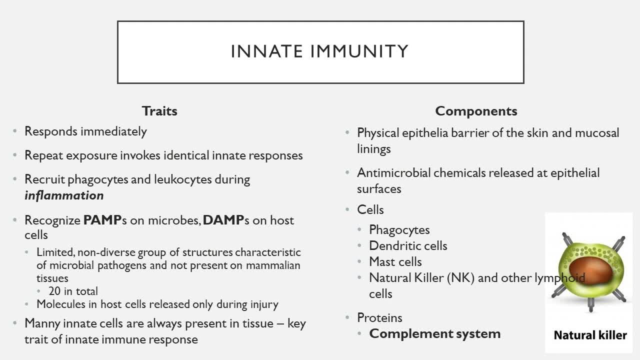 are a group of limited, non-diverse group of structures that these recognition receptors can recognize. So these are things common to bacteria, viruses and fungi, And there's only about 20 or so of these different molecules that these pattern recognition receptors can recognize. 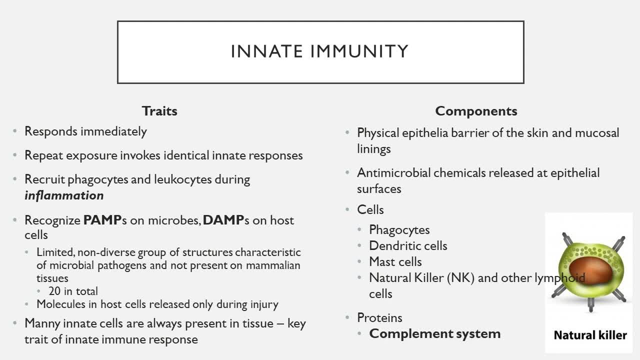 So it really highlights the low diversity of these PAMPs. The damage-associated molecular patterns are found in host cells, but they're only detectable whenever cell injury has occurred. So there's always a risk that the immune system is exposed to these PAMPs. The PAMPS will not be. 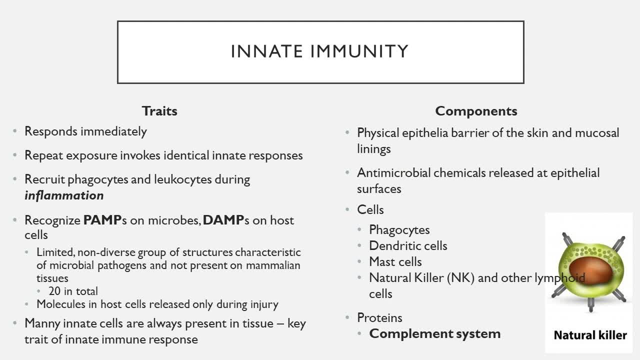 able to recognize the PAMPs. So one of the reasons that these PAMPs can be recognized is because they are in the extracellular fluid. If you look at the orange line on the left, it's the cell wall, the lipid bilayer, And whenever a cell gets disrupted through necrosis and note, not apoptosis- 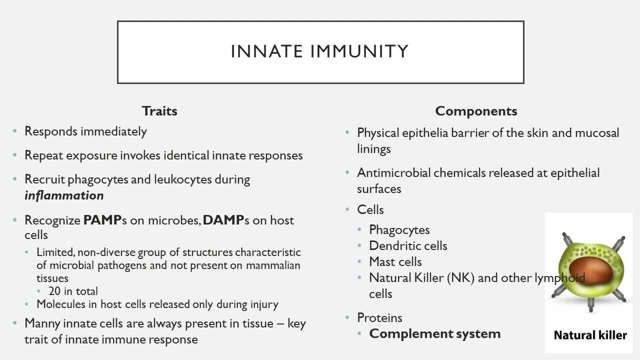 these patterns get released And then that way, when they're in the extracellular fluid, then cells of the innate immune system can recognize them and it triggers alarms. Now, one of the reasons why the innate immune system can respond so rapidly is that many innate 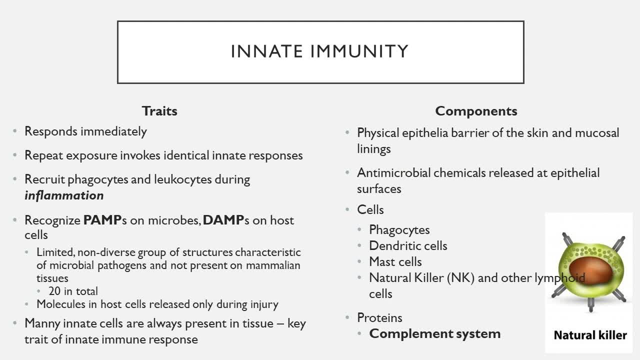 abundant in our bloodstream, They're the most common leukocyte, So they're always around, they're systemic and that's why they're always on site to respond rapidly. Now, the four main components of the innate immune system isn't just limited to cells, There's a physical barrier. 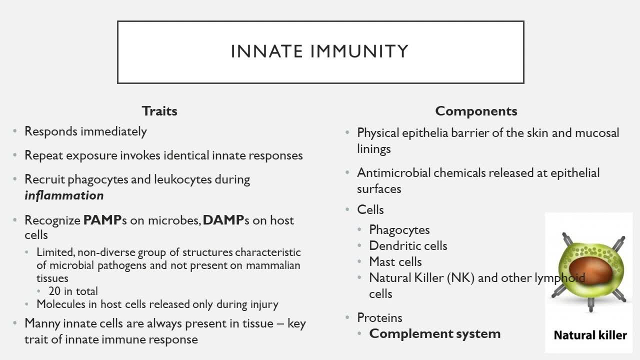 which is the epithelial barrier at our skin and mucosal linings that keep out pathogens, And this is the part that gets compromised when there are cell injuries, like through surgery and the implantation of a biomaterial. There's antimicrobial chemicals, So there's a chemical barrier that 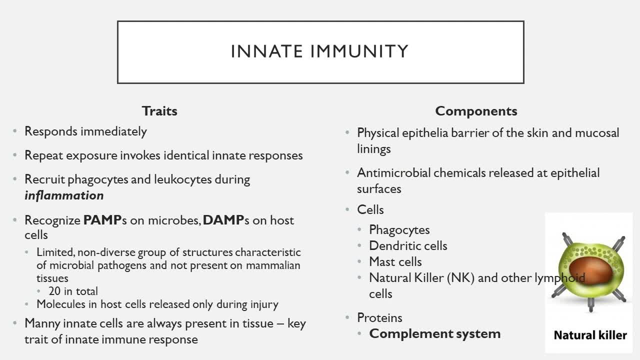 are either constitutively present or released at the epithelial surfaces. so our stomach lining, our mucosal linings, have natural defensins and chemicals that fight against pathogens. Cellular-wise, there's a number of different cells that are involved in innate immunity. There's the 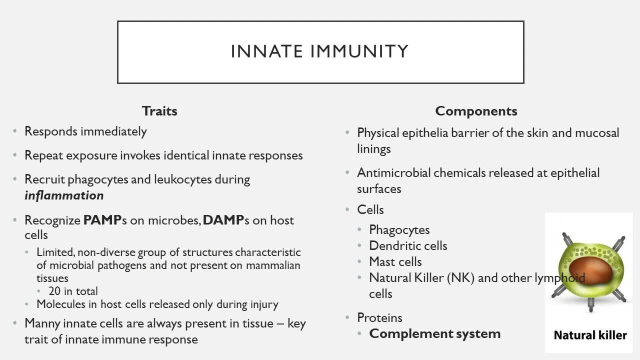 phagocytes we'd already discussed, which include monocytes, macrophages and neutrophils. Dendritic cells are perhaps some of the coolest cells, I think, in the immune system, because they help bridge the innate immunity, adaptive immunity. We won't talk about them too much here, though. 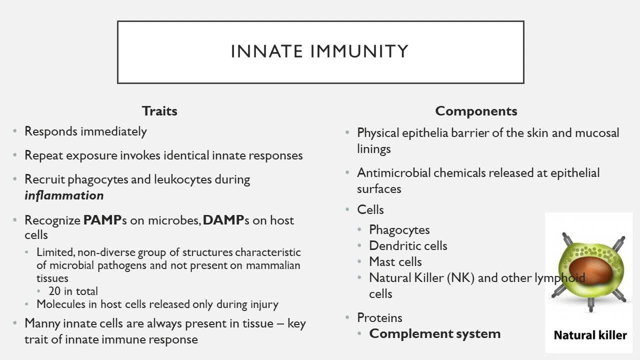 Mass cells are granulocytes that have these chemical payloads called granules, which is what gives them their needs within the cell. cytosol And these payloads of chemicals get released during inflammatory reactions and can cause irritation. They can increase the inflammatory response And this 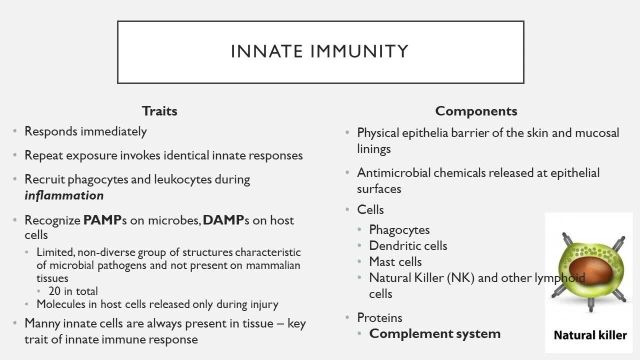 is the primary mechanism that actually drives allergies. So a lot of times, when our body responds to benign foreign materials that get triggered by mass cells to degranulate, we see the symptoms of these degranulations And then finally there's natural killer cells. 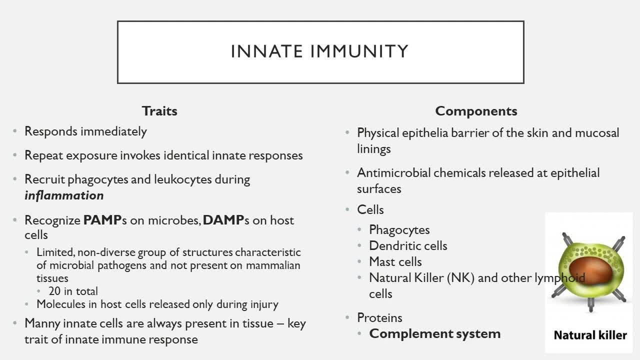 And other lymphoid cells which help attack against viruses and bacteria in nonspecific ways that contrast it to the adaptive immune system. Lastly, there's proteins such as the complement system, which is sort of the innate immune system's response to antibodies in the adaptive 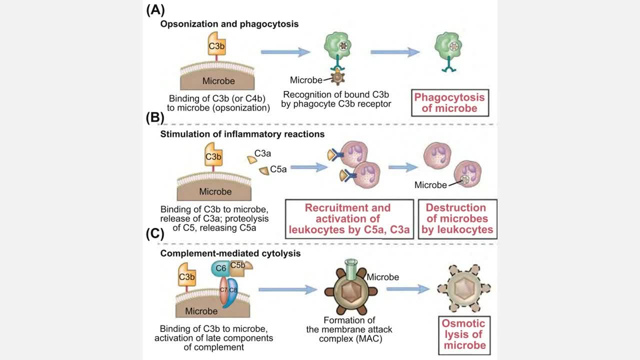 immune response. The complement system is interesting and I think it often gets overlooked because it doesn't have too many primary functions itself that it directly carries out. It usually is in helping roles. It complements the roles of phagocytes, antibodies and other cells in the immune system, which is 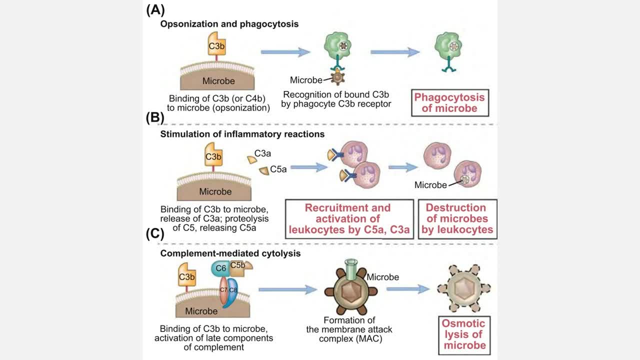 what gives it its name. So I just want to quickly go over a few of the functions and then we'll move on from there. So complement proteins are great opsonizers, which means that they coat bacteria or viral cell walls. They help phagocytes recognize them. So sometimes, when 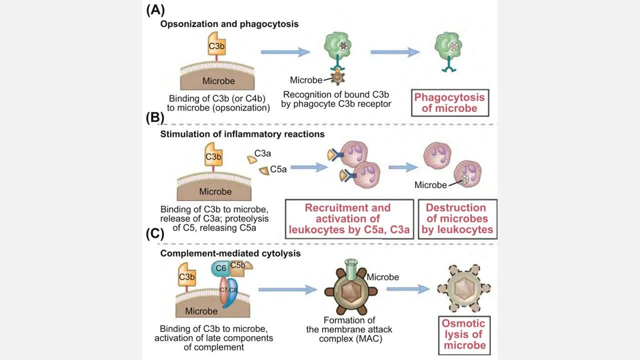 cells can't recognize pathogens directly. what they do actually recognize are complement proteins that have stuck to the walls of these cells. So they stick the walls in those complement receptors on phagocytes that recognize them, and that's what initiates phagocytosis, as opposed to these phagocytes recognizing the 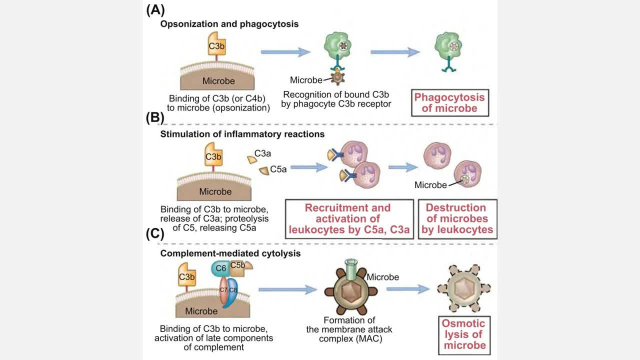 pathogens directly. I often think of complement as this cascading series of proteins that bind to cell walls. they get cleaved, they create new protein complexes that cleave other proteins and it keeps in, this continuing cascading reaction that builds up of both proteins on the cell. 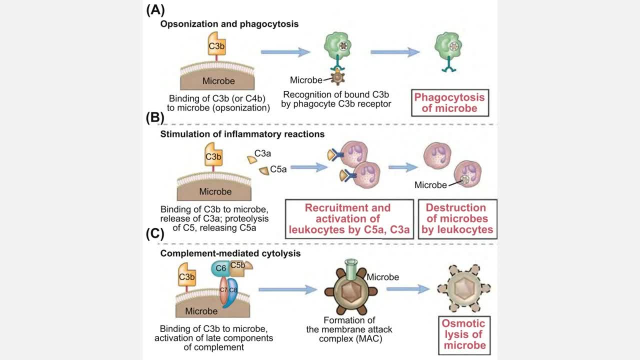 wall and these fragments. So when we start to look at these complex components, it will often be produced by an immune system. So fast forward to this one. so in this case, I'm going to produce a product which is a new phagocytes stimulant that takes out the immune system from the cell wall and creates 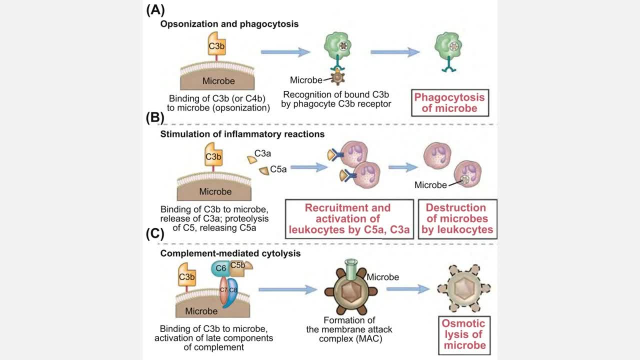 new of theseolanes, the immune system. So if you look here, you can see the membrane which is formed by the phagocytes and there's a structure called the immune system And it comes from our cell wall. It's a structure called the immune system. 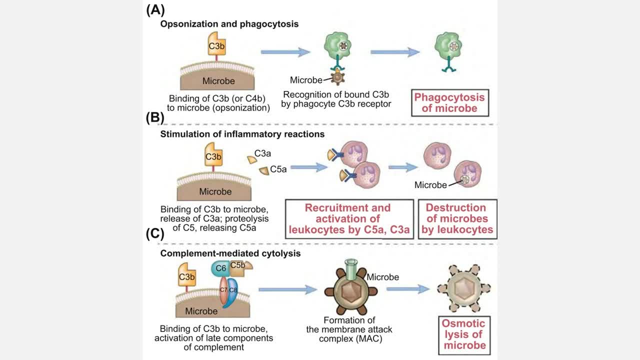 of initiating cytolysis or lysis of bacteria and pathogen cell walls. I mentioned before that it's a cascading reaction. Well, whenever these proteins start clumping up, eventually they get so clustered and so dense that they literally rip apart the cell walls of bacteria and viruses. 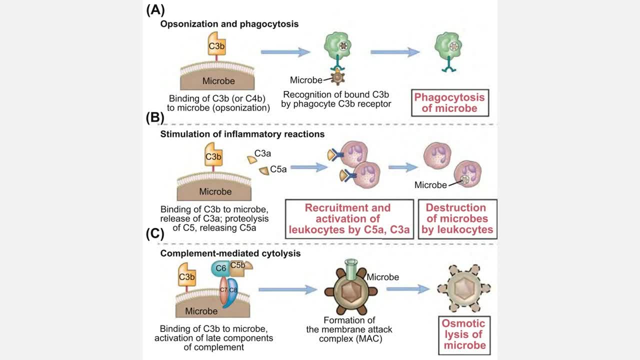 and they create these huge pores that allow the influx of extracellular fluid, which eventually results in lysis of the cell. Now, in short, what I want you to take away from this is that complement gets activated whenever it recognizes a foreign wall. It can only attach to things that 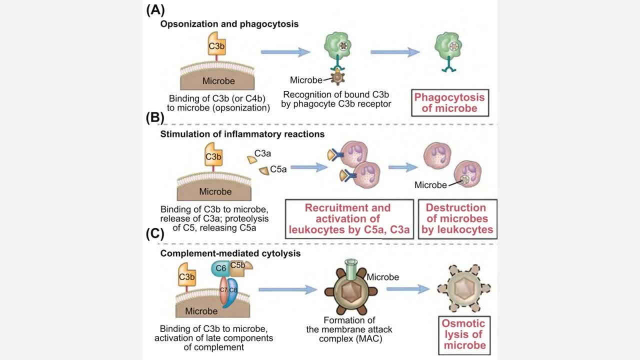 are foreign to the body, Our own cells have natural ways of hindering and inhibiting complement activation, but whenever it encounters a foreign wall, like with a pathogen or with a biomaterial, that initiates this cascading reaction that can instruct phagocytes to try and phagocytose a. 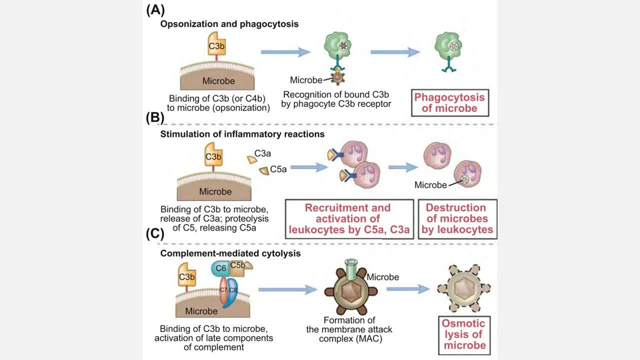 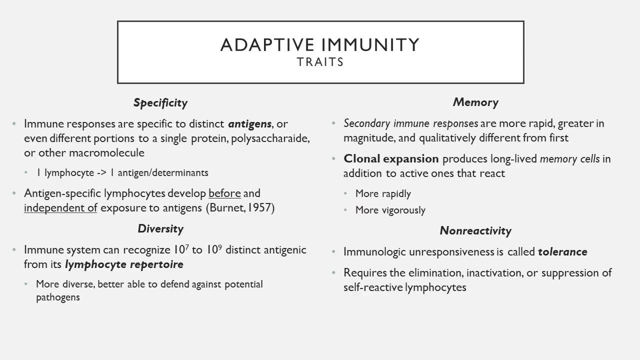 biomaterial. It can also stimulate the inflammatory response and cause for the recruitment of leukocytes and monocytes. Now, adaptive immunity has a few traits that really contrast it with innate immunity, The first one being specificity. So, in contrast to macrophages and neutrophils, which are all 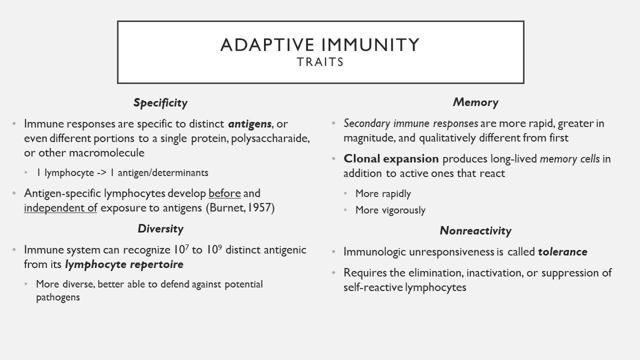 identical to each other, or at least there are specific subtypes and what they respond to. lymphocytes of the adaptive immune response are highly specific, And one B cell that recognizes a very specific part of an antigen, something that it binds to. 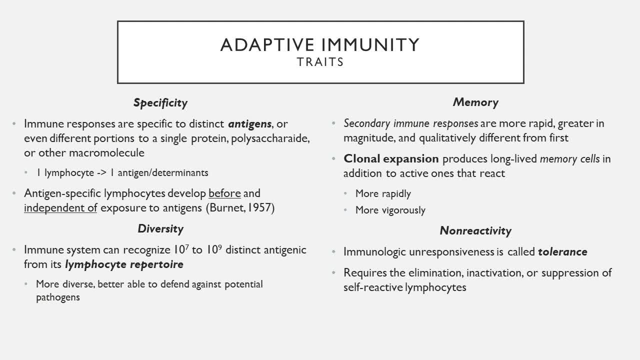 would be very different from a near-identical B cell that just has a different specificity. So all these B cells are coded differently from the start and every lymphocyte has only one job, and that's to recognize one specific thing. So they don't have the same broad recognition. 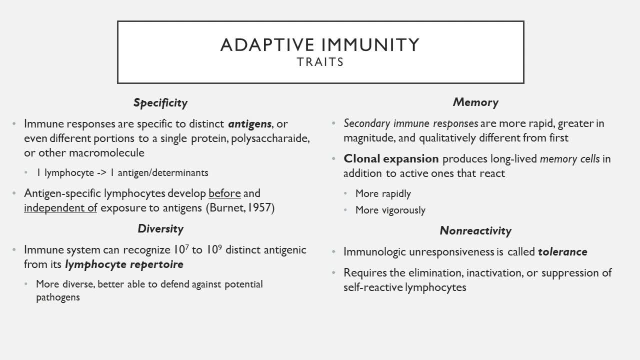 capabilities as cells of the innate immune system. Along with that is their diversity, right? So I mentioned before that pathogen and damage-associated molecular patterns. there's only about 20 of them or so that cells of the innate immune system have, So there's only about. 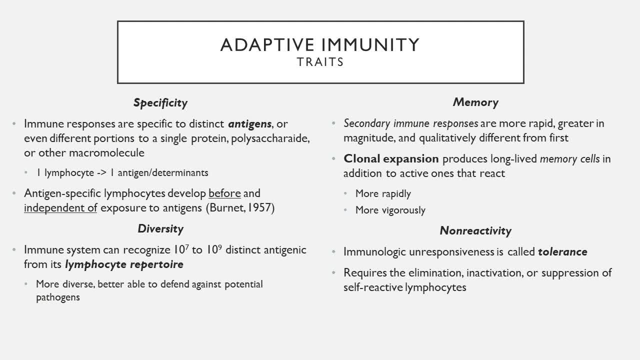 20 of them or so that cells of the innate immune response can recognize in this sort of broad fashion. So they have very limited diversity of what they can recognize. So the adaptive immune response, however, can recognize and differentiate 10 to the 7,, 10 to the 9 distinct antigens And 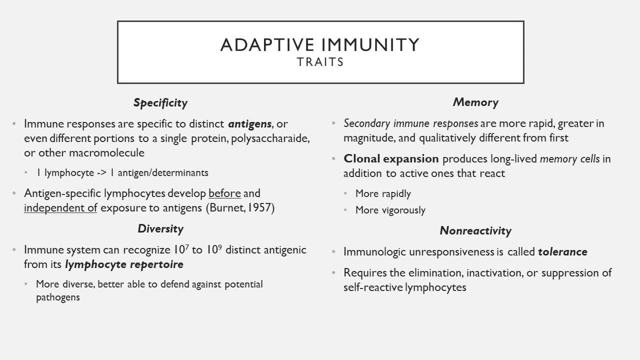 this is what's referred to as the lymphocyte repertoire. Now again, to differentiate this from the innate immune response: repeat exposures to macrophages and neutrophils or other cells within the innate immune system doesn't elicit any greater or lesser reaction from those cells. 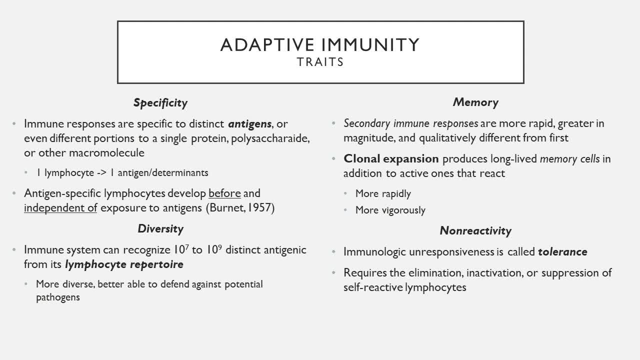 They have no memory of it. They don't respond differently. It's just as if they're responding to the first time. every time That's different. in adaptive immunity We can train ourselves to respond to something, particularly if it's bad, so that secondary and third responses are. 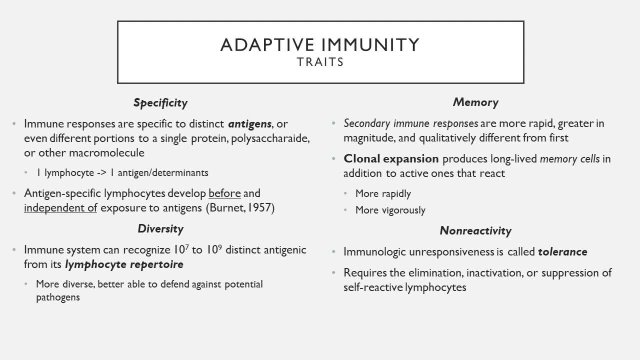 much more benign, in part because we're so much better and capable of fighting off against it, And this is the real principle behind immunization: We can train our body to react with something in a nice, controlled manner, and that way we don't even recognize it whenever we're fighting off. 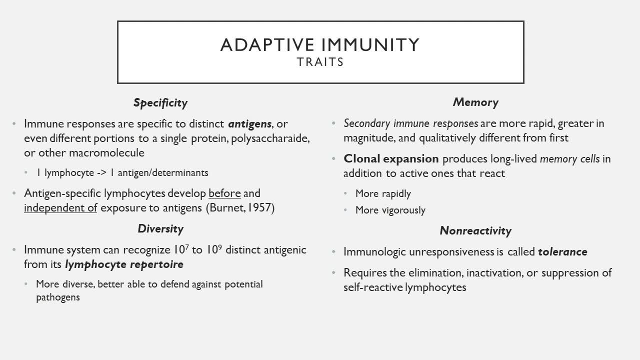 that same pathogen. So we can train our body to react with something in a nice, controlled manner, and that way we don't even recognize it whenever we're fighting off that same pathogen or bacteria the second or third time. So it's very common, of course, that you encounter pathogens all. 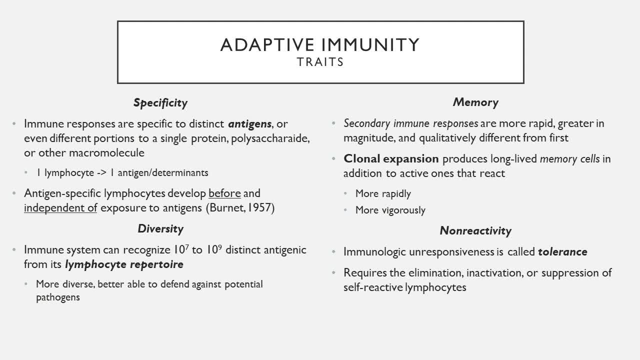 throughout the day. It's just the fact that we've been exposed to them previously that makes it such a benign response. Part of what causes this is the idea of clonal expansion, where, after we've been exposed to something, our body produces from one of those single lymphocytes that were 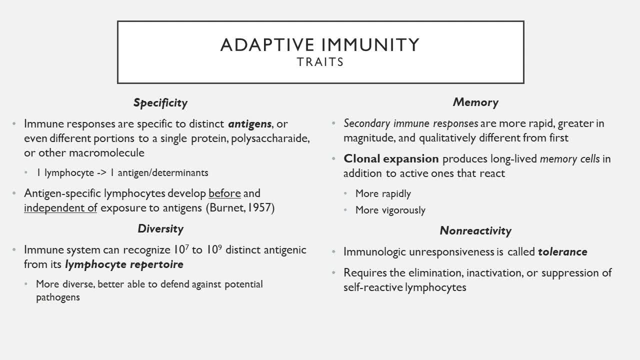 initially diverse and specific. against that, one pathogen produces tens and hundreds of thousands of cells of that same original copy And in doing so produces memory cell versions of that original naive cell prior to exposure. And it's these memory cells that are trained to respond faster and more rigorously upon repeat exposures. 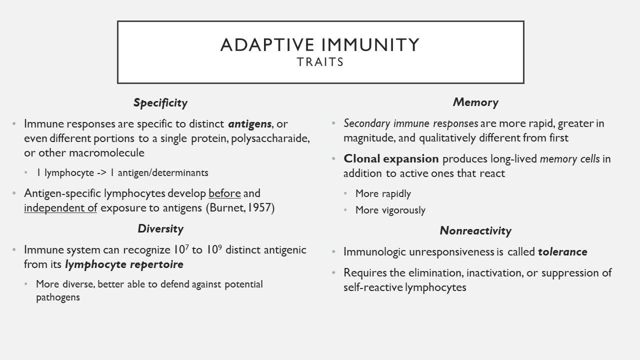 to produce again that army necessary to fight off against these pathogens. Now, the last trait has to do with non-reactivity. Whenever our cells produce these lymphocytes that are so distinct and so specific, it is possible that we accidentally produce cells that are reactive against. 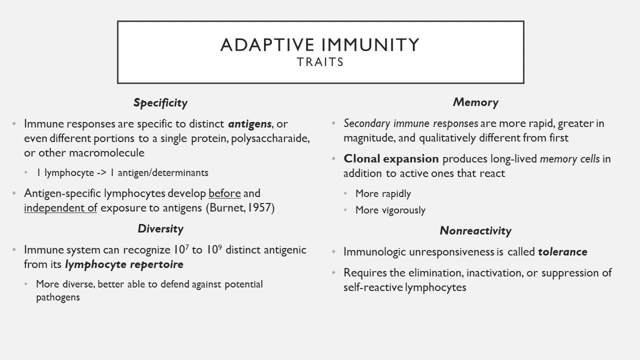 our own host cells And then our body actually has mechanisms where we sort of train these cells and give them exposure to our own host cells and control its ways so that whenever they recognize them we see that there's self-reactivity and then your body quickly gets rid of that lymphocyte so that it doesn't. 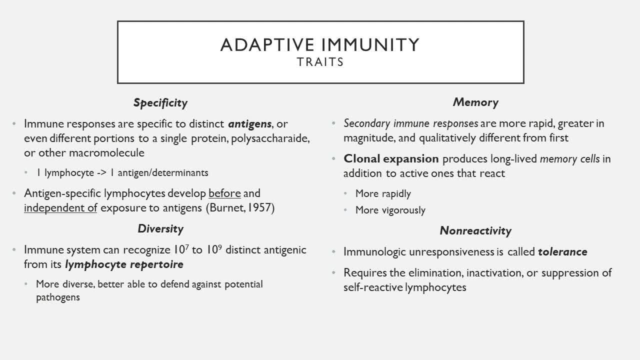 actually enter circulation or the lymphatic system where it could possibly react against more cells within us, And this is the idea of tolerance. So we actually train ourselves to be tolerant of our own cells and we get rid of lymphocytes that would potentially respond to these cells, And so we have to. 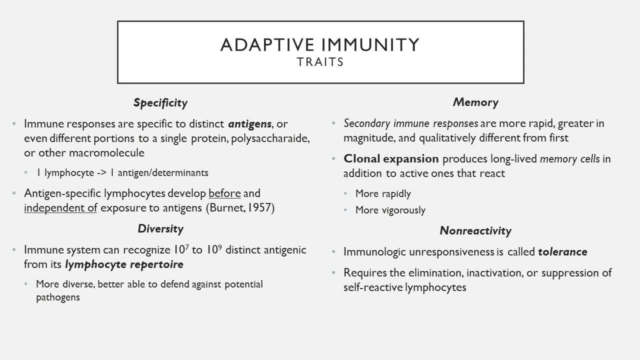 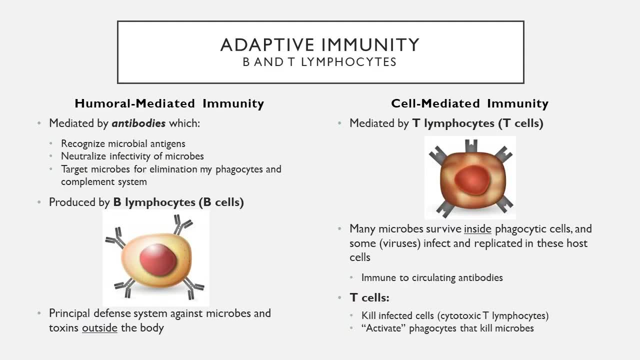 react against them, And so whenever this mechanism of tolerance fails, that we have autoimmune diseases. Now realize all throughout the last slide I kept saying this word, lymphocytes, and never did a proper introduction of what lymphocytes are. So lymphocytes are a type of leukocytes. 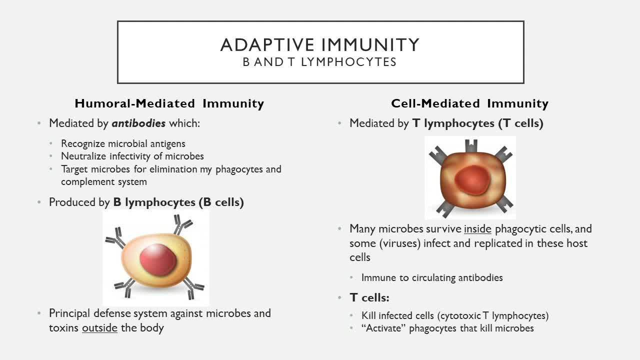 in which T cells and B cells fall under. Now these are both key cells involved in the adaptive immune response. Now B cells are involved in the humoral mediated branch of adaptive immunity. This branch is the principal defense mechanism against microbes and toxins outside the body. 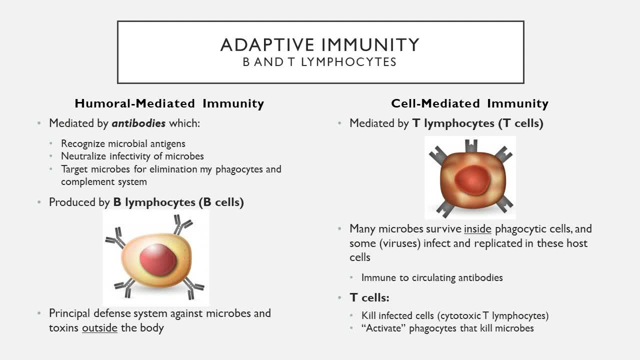 within adaptive immunity. And the real key player again is B cells. They're the factories that produce what actually mediates the effector mechanisms of this branch, which are antibodies. So B cells are factories, They produce antibodies, Antibodies. they can recognize a diverse and 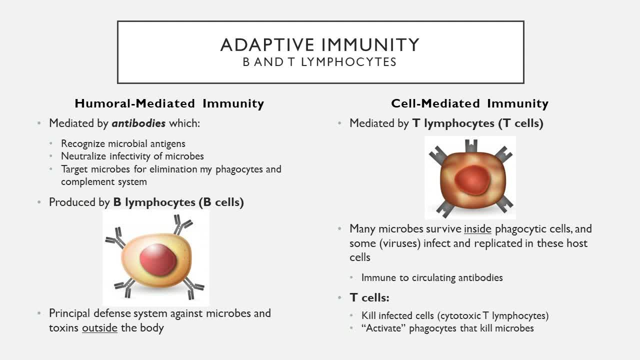 highly specific amount of molecules, whether they're associated with pathogens or not. They can neutralize pathogens and toxins Simply by bonding to them. And just by bonding to them they can prevent pathogens or toxins from either binding to receptors of our cells, infiltrating 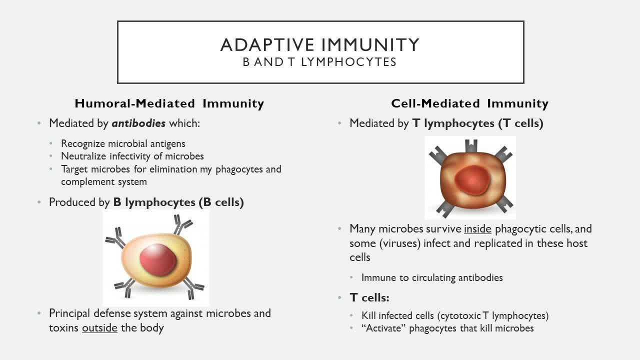 our cells migrating around the system and just keeps them from doing anything And eventually they're just cleared by the body through natural mechanisms. They can also target microbes for eliminations by phagocytosis and the complement system. So they work. with complement They work. 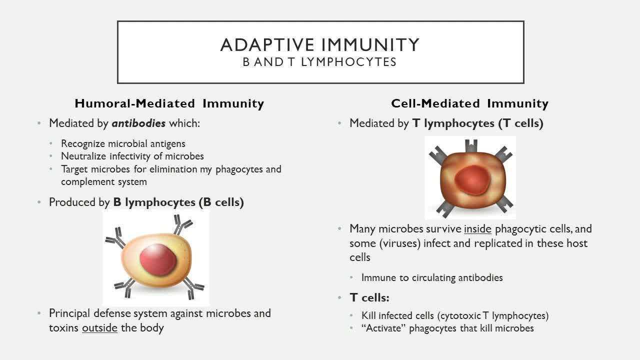 with cells, the innate immune system. They are fantastic opsonizers, both in part because they can bind so strongly to pathogens or bind to the immune system, And they can also bind to the biomaterials And also they're specific against them. So again, antibodies are used to fight off. 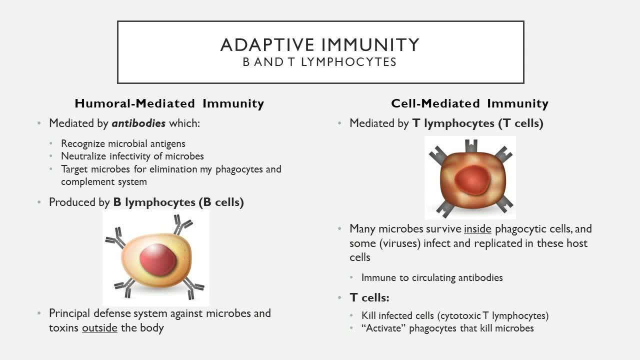 against things outside of host cells. Okay, if they're floating around the extracellular space, if they're in circulation, antibodies that are in circulation can get access to them and bind to them. But if a virus or bacteria somehow infiltrates a host cell and affects it, antibodies can't get. 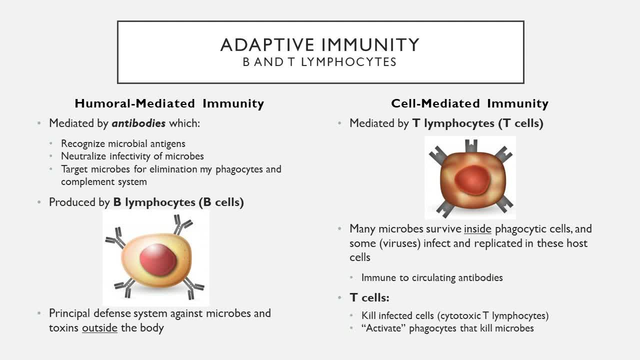 inside our own host cells to perform their effector functions. This is why we need T cells. So a lot of viruses love living inside cells. A lot of bacteria do as well, And they can't be eliminated by phagocytes on their own, And this is why we need T cells. So T cells can come in two different branches. They can help. 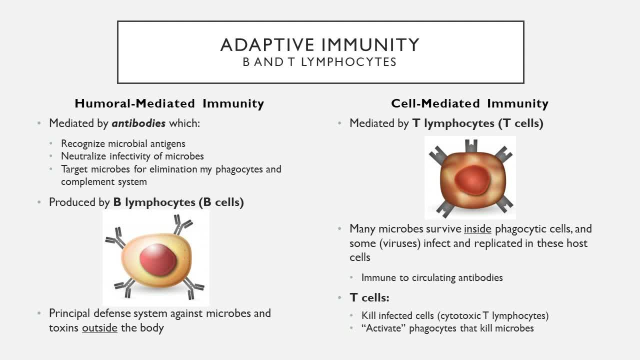 phagocytes perform out their jobs much more effectively. They can also come in cytotoxic T killer cells which instruct the infected cells to commit suicide, thus killing the viral replication mechanism. So again to contrast the two different lymphocytes B cells produce 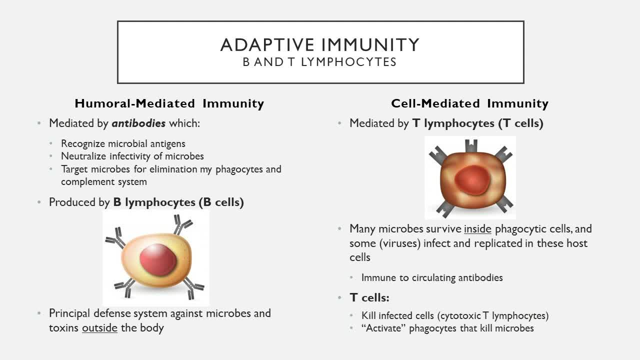 antibodies, and it's antibodies that mediate functions for defenses against microbes outside of cells And it's T cells that directly mediate the functions against pathogens inside of cells. So I thought that was a good overview of both the innate and adaptive immune system. The innate immune response admittedly comes into play a lot more. on the 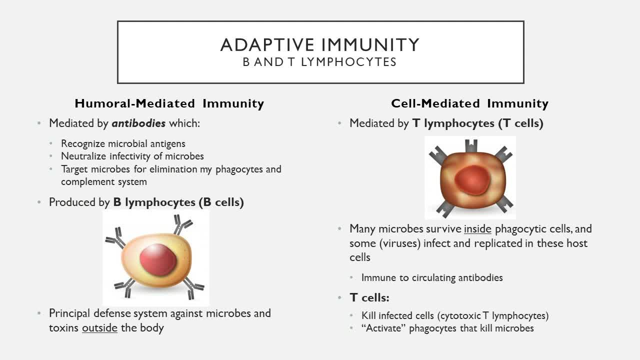 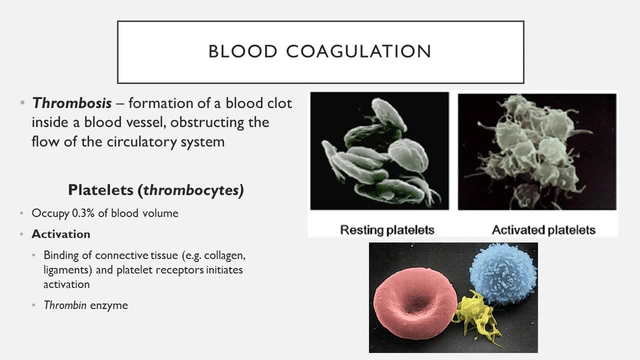 focus of biomaterials, because lymphocytes can't recognize, or aren't trained to recognize, patterns associated with non-living materials. So the last portion of this lecture is going to focus on the coagulation process and the cells and proteins involved in that. Now, coagulation is just the 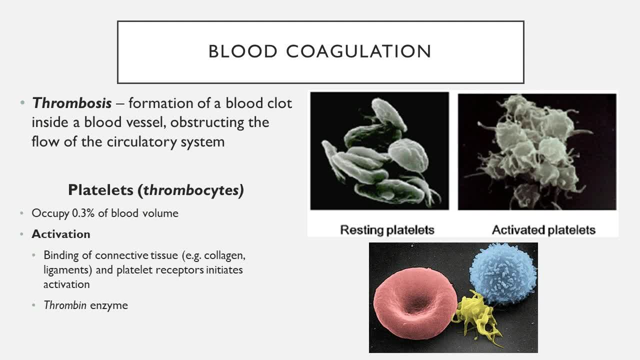 general clotting of blood. Thrombosis is the formation of a blood clot inside of a blood vessel, which can obstruct it and obstruct the flow of the circulatory system. Obviously, the goal in developing a biomaterial, especially one that has blood-material interactions, is to prevent. 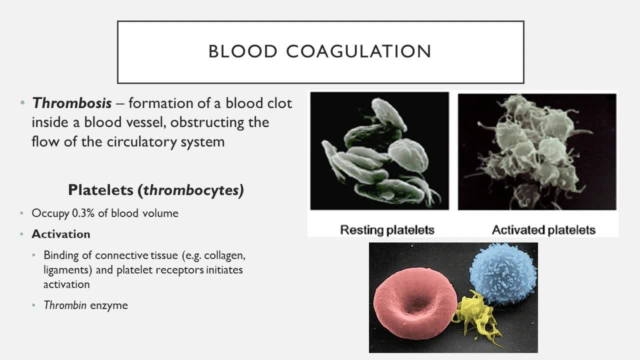 thrombosis or embolisms, which is the breaking off of blood clots that can go downstream and potentially block something away from the site. The main player in thrombosis are platelets, which are actually called thrombocytes for this reason. They're a leukocyte that occupy only 0.3% of blood volume And they can go from this resting. 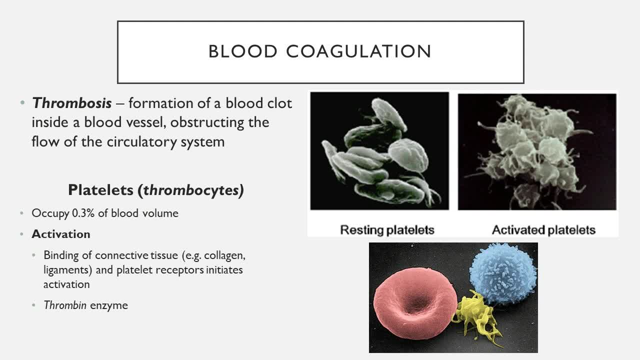 state to inactivated state very quickly. They're very finicky and involves binding to connective tissue like collagen. Collagen is a fantastic initiator of activation, In part because you can imagine, collagen is not part of the endothelial blood vessel lining. It's not found within the 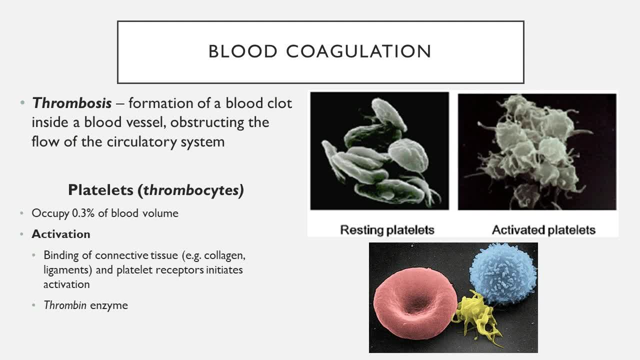 circulatory system. So the only way to do that is to activate the blood vessel lining. So the only way that a blood cell or a platelet would find it is if there was some sort of injury that caused blood to flow into non-vascular areas. Another key player which we're going to find out a little: 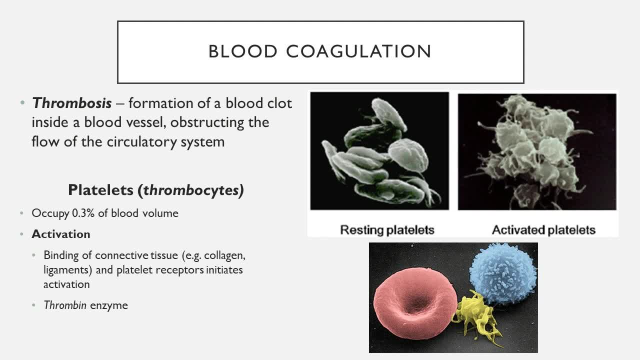 bit more soon is the thrombin enzyme that not only initiates activation, but also progresses it through the coagulation process. So now let me play this YouTube video on platelets and the coagulation process, and then we can talk about it a little bit more in detail. 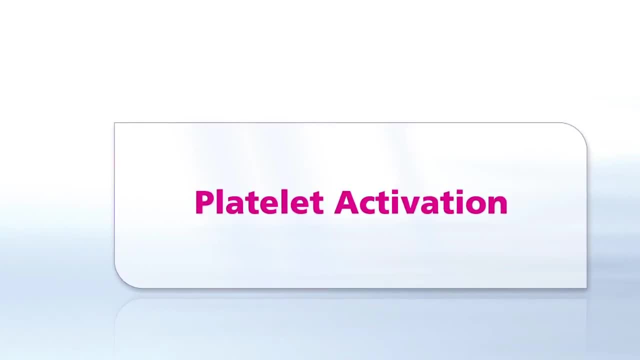 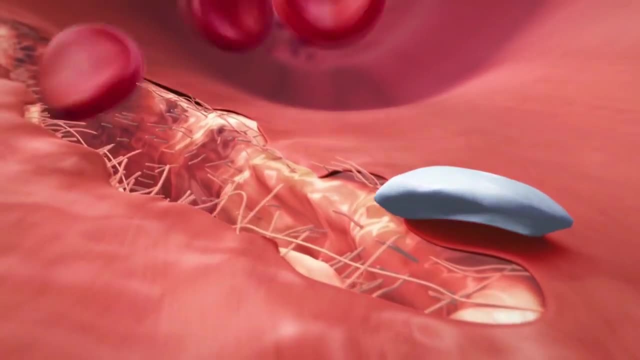 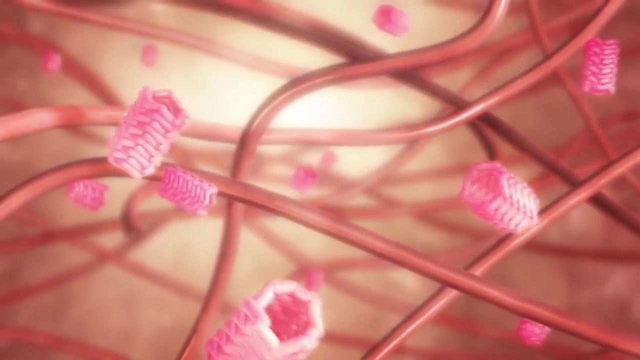 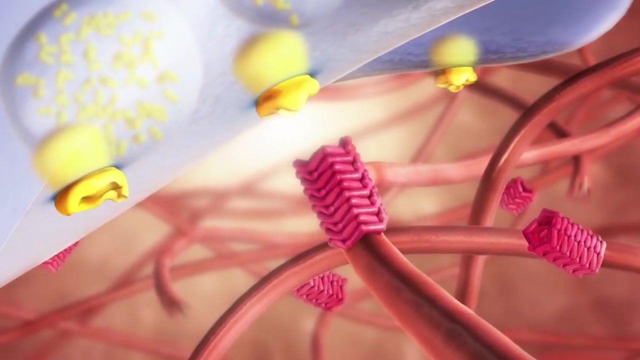 In a first step towards clot formation, platelets are recruited to the site of vessel injury by now exposed molecules of the vessel wall, such as collagen and von Willebrand factor. This factor mediates the linking of platelets to collagen via a specific receptor in the platelet membrane. 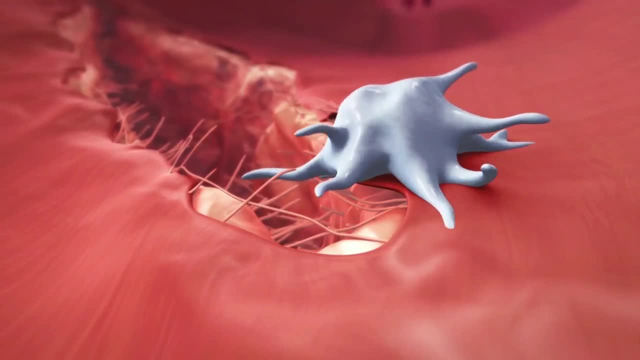 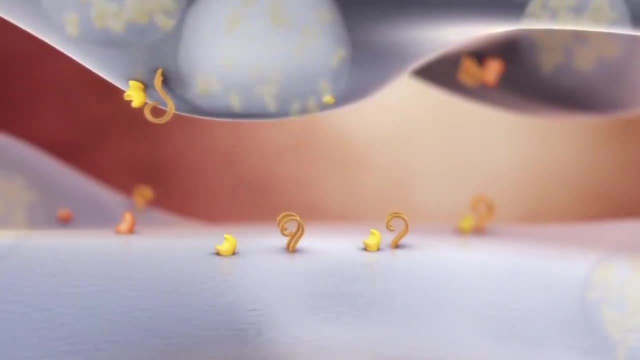 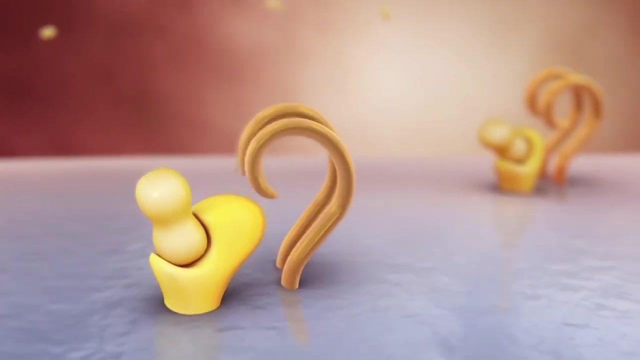 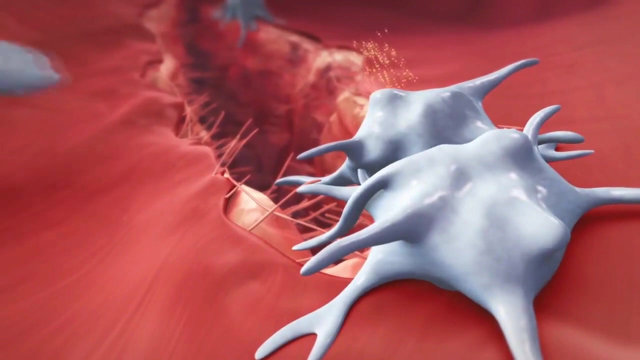 The resulting change of shape of the platelet from its resting state into the dendritic form indicates activation. The activated platelet in turn releases prothrombotic molecules such as adenosine diphosphate, ADP. By binding to its receptors, ADP induces aggregation and recruits further platelets to the site. 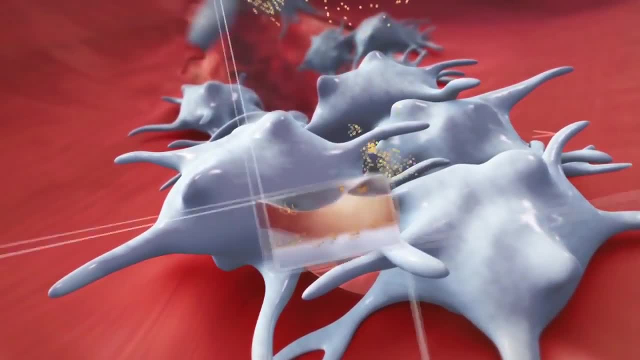 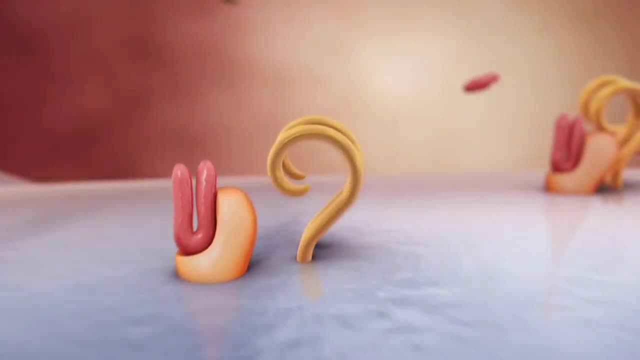 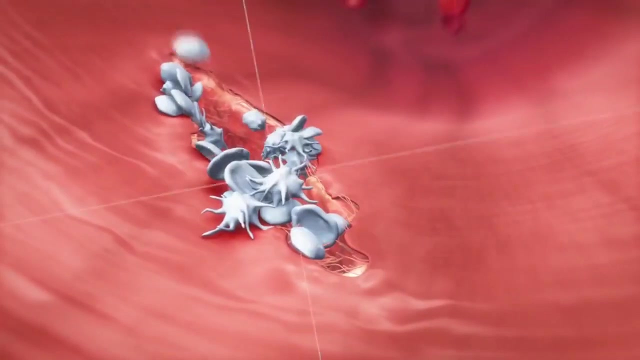 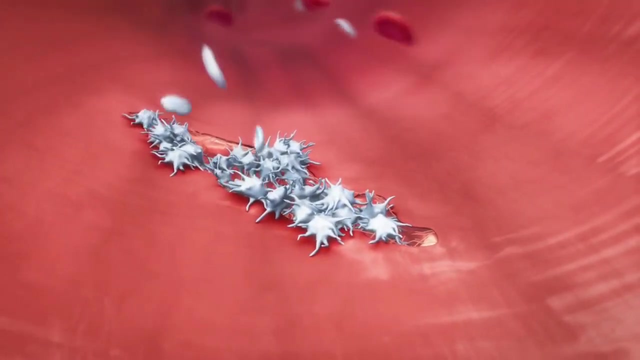 thrombocsine is another important mediator of platelet activation and aggregation Until later cells. under its influence, the platelets cross-link with each other. These interlocking mechanisms cause platelet activation. to snowball, The clot grows rapidly. Activated platelets also trigger the coagulation cascade and thus the formation of thrombin. 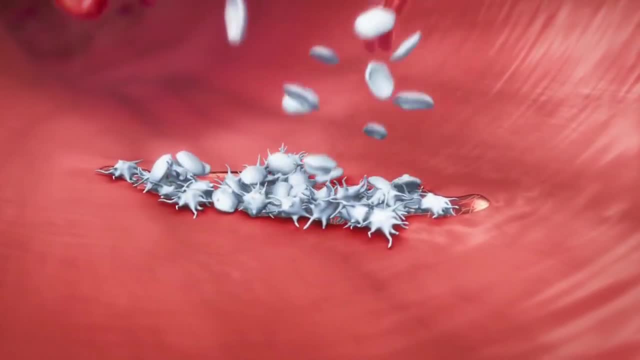 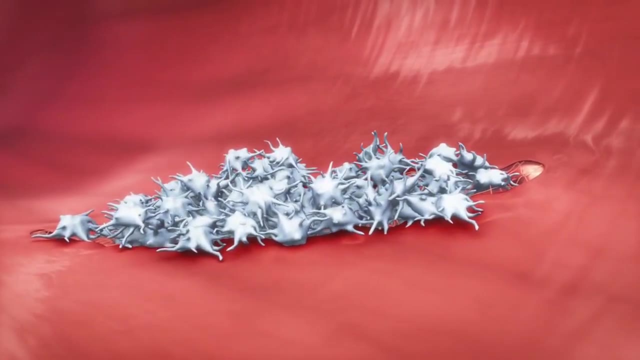 Mist 줳� 대 thrombin. homeland Trombin in turn stimulates platelet activation even further: a continuous feedback loop. Additionally, thrombin induces the formation of fibrin for the mesh, stabilizing the clot, The self-reinforcing process of platelet. 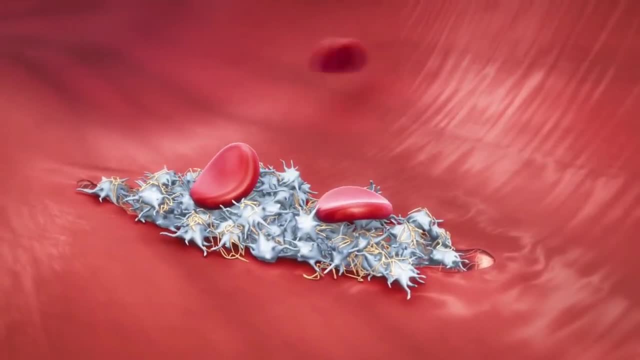 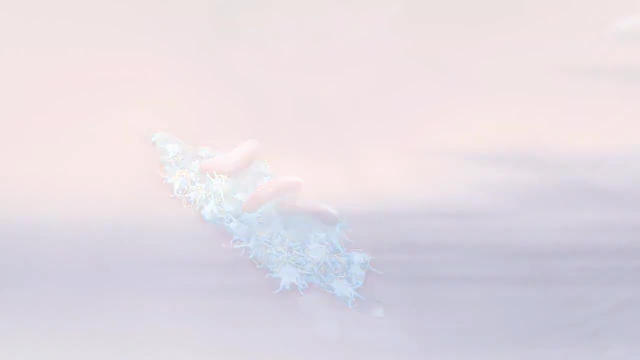 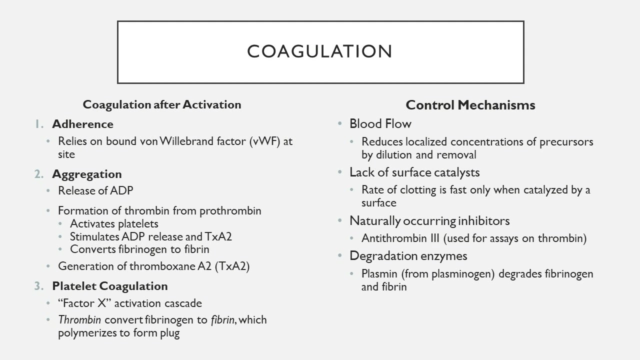 activation, crucial in the formation of blood clots, is an obvious therapeutic target in conditions caused by inappropriately triggered blood coagulation. So I thought that was a fantastic overview of the entire coagulation process, So let's dive into it in a little bit more detail. So, as I said, 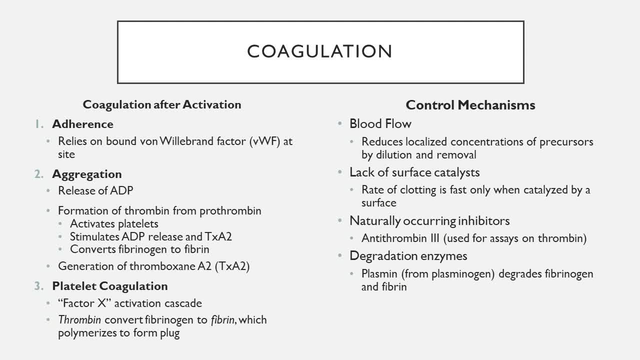 platelets are really finicky and extremely sensitive cells that respond to minimal stimulation and after this activation that platelets changed their shape from a nice sort of like squashed shape to a sort of like squashed shape, That platelets have thin, low and thick color. These platelets are really five and five inches long. 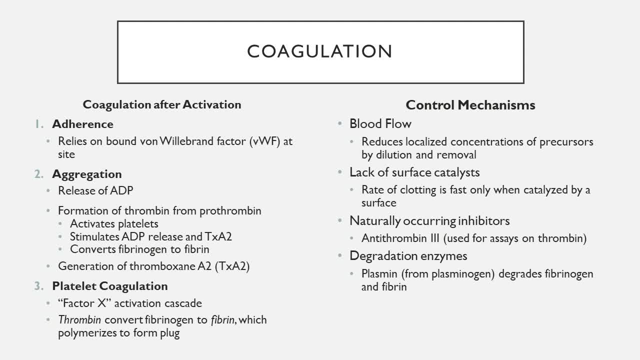 circle into this really spindly shape that allows for adhesion to occur. So this is after activation. Adherence relies primarily on the von Willebrand factor adhesion protein. Now, it's important to know that von Willebrand factor isn't just an adhesion protein in this case, but also 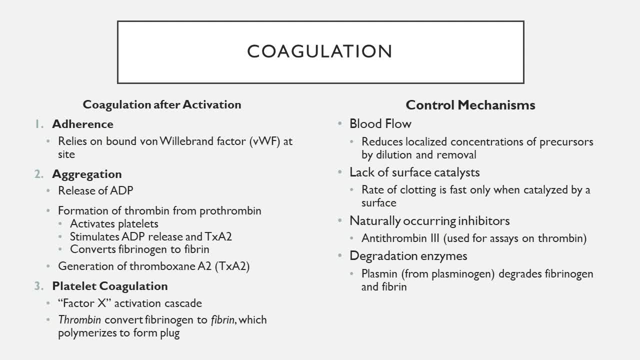 a cofactor that acts as a surface receptor for platelets to continue this activation coagulation process, And the importance of this can be observed in patients that have genetic diseases that lack this receptor for von Willebrand factor, that suffer from serious abnormal bleeding in case of injuries. Now, following platelet adhesion, there's a complex 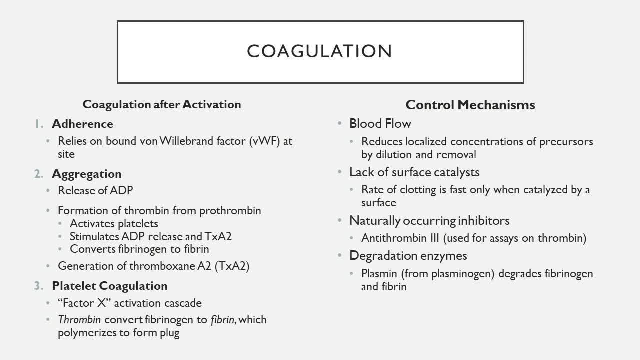 series of reactions that's initiated by the release of three primary chemicals. So one is ADP, adenosine diphosphate, The other is the formation of thrombin from its precursor, prothrombin, And then the third is the generation of thromboxane A2.. These are all released by the. 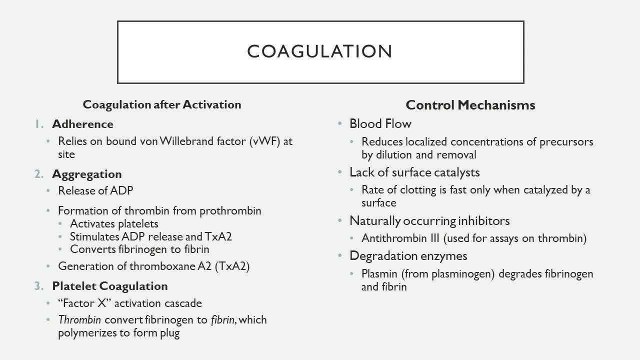 adhered platelets That cause further activation of non-activated, non-adhered platelets that continue this adhesion process. So it's the sort of pro-feedback mechanism that causes cascading reaction of coagulation. This is all mediated by thrombin itself and that thrombin promotes further release. 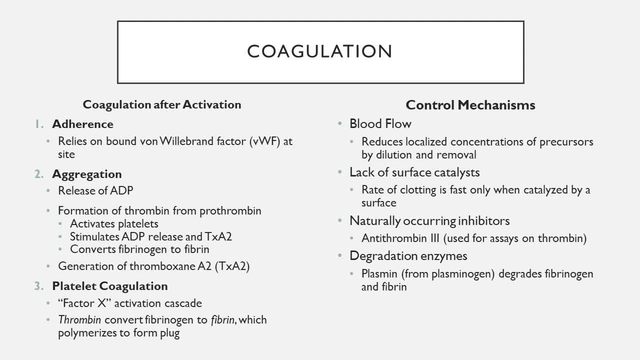 of ADP and thromboxane. It also converts the precursor fibrinogen into fibrin, which is really what is the glue that keeps all these activated and adhered platelets together. So it's said to be one of the most important proteins supporting. 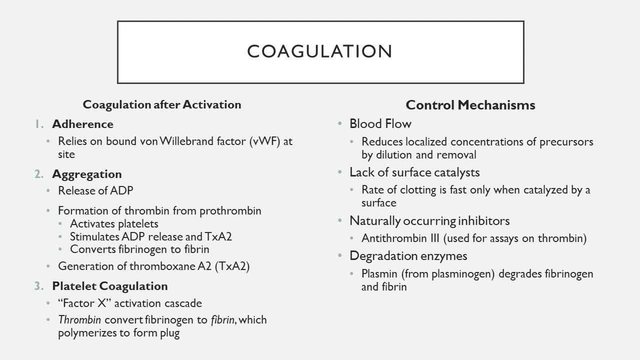 platelet adhesion of fibrinogen. Now, that all describes the aggregation of platelets. The actual coagulation process is the formation of that fibrin glue that polymerizes and entraps all those platelets into a sort of like an extracellular matrix, And it relies on two things. 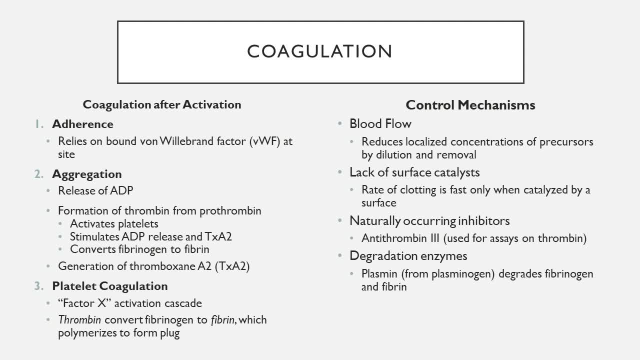 that all kind of lead into fibrin. Factor X is an activation cascade. that was really just a series of mechanisms that form a sequential pattern, in the same way, I kind of think, as the complement pathway, And they all serve to eventually convert prothrombin into thrombin. And then, lastly, it's 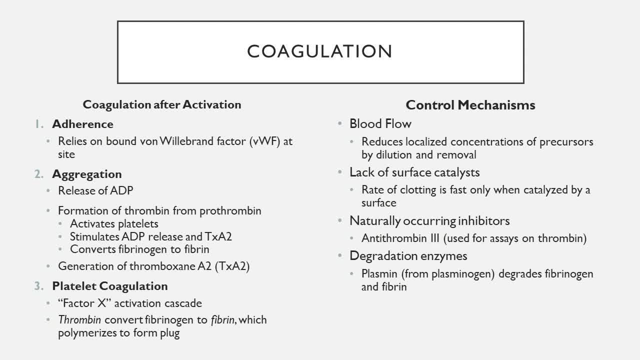 the thrombin that converts fibrinogen into fibrin, which, again, I described as the glue that holds all the aggregated platelets together. Now there's a number of inhibitory or control mechanisms. the body has to always keep coagulation in a control because it's actually an ongoing process within. 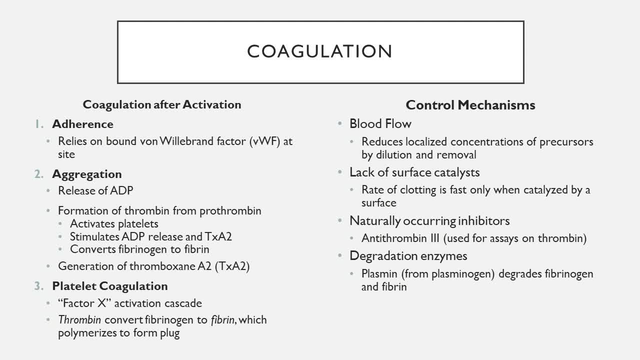 our body, And it's a process that we're going to see in the next couple of weeks. So we're going to talk a little bit more about that in just a few minutes, But before we do that, I just want to remind you that we're going to talk a little bit more about the flow of blood, that we just are. 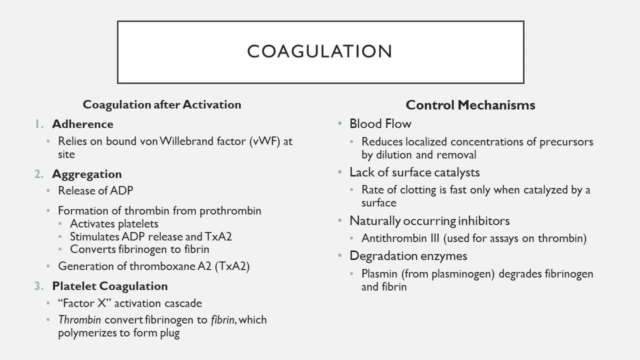 really adept to inhibiting. So one of those main reasons is actually blood flow. So the flow of blood actually reduces the localization of all the enzymes and proteins necessary for coagulation to occur, And it's only whenever there's a site of injury or a break in blood vessels where blood is 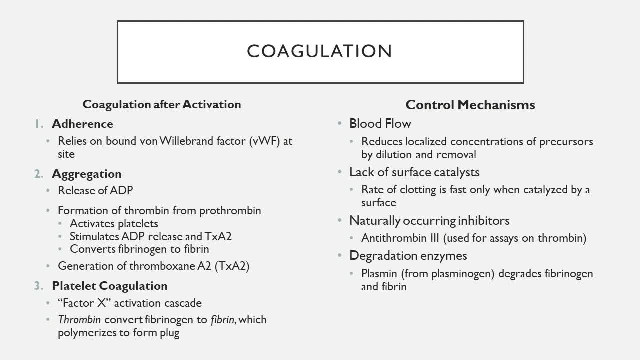 allowed to pool and then just aggregate and continue reacting in one spot, as opposed to being distributed systemically. There's also a lack of surface catalysts, So they're all going to need to be something that initiates the initial activation and adherence And our body's 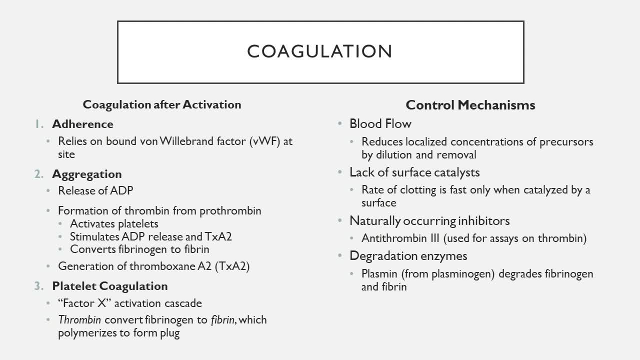 blood vessels. the endothelial lining is just really good at preventing that, And it's only whenever blood comes into contact with unnatural materials or ones outside of the circulatory system, like collagen, that this can actually be initiated. Surfaces also have naturally occurring inhibitors, So even ones that do start a minor adherence process can actually inhibit it, And that's what antithrombin does. In fact, we use antithrombin to inhibit blood vessels. So we use antithrombin to inhibit blood vessels, And that's what antithrombin does, And in fact we use. 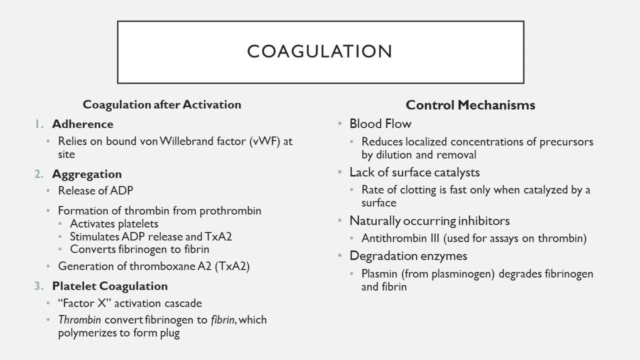 antithrombin to inhibit blood vessels, And that's what antithrombin does, And in fact, we use antithrombin and combinations of throbbing and antithrombin that bind together as assays to determine if a material is likely to cause coagulation. have adverse events related to? 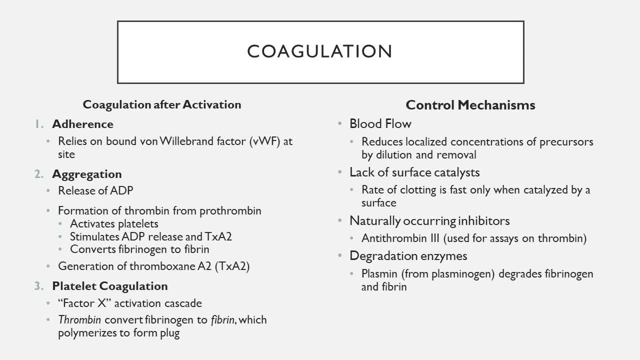 blood material interactions. Finally, there's degradation enzymes that, instead of blocking the initial adherence or aggregation process, actually degrade the blood clots and coagulations that have already formed. Plasmin is a great example of this type of enzyme. It comes from 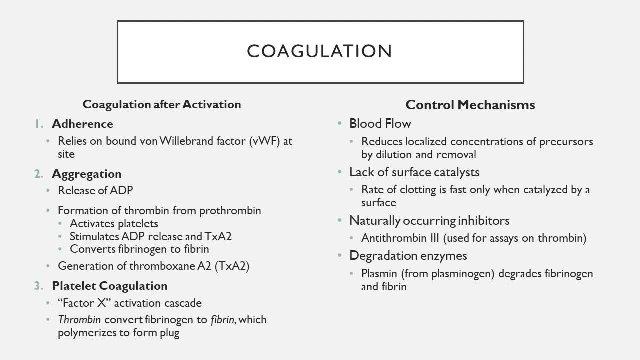 the precursor plasminogen, and this degrades fibrosis, And it's a great example of this type of enzyme. It's a great example of this type of enzyme. It's a great example of this type of enzyme: fibrinogen and fibrin- again, the glue that holds these platelets together. 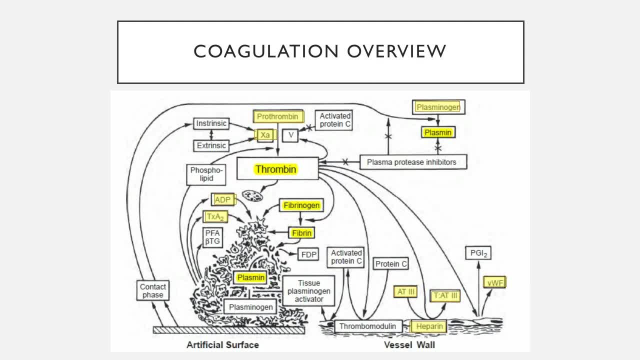 Lastly, I think this chart is a great overview of the coagulation process and the inhibitory mechanisms that prevent coagulation or aggregation from happening in the first place. So on the left you see a natural, a blood clot that's formed on an artificial surface. That clot is giving up. 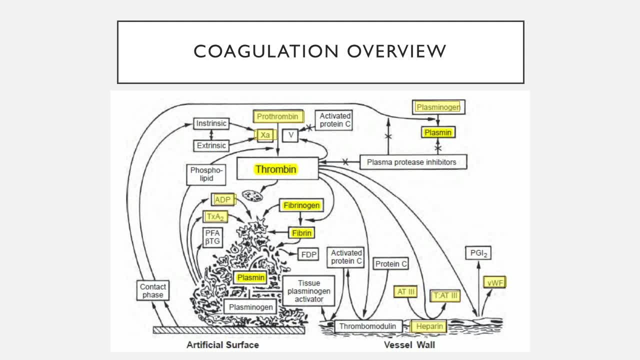 thromboxane, which is the TXA2, ADP. It's helping to convert prothrombin into thrombin through the factor X cascade. Thrombin in itself is converting fibrinogen into fibrin, which again is part of the glue that holds all these platelets together. Within that there's inhibitory. 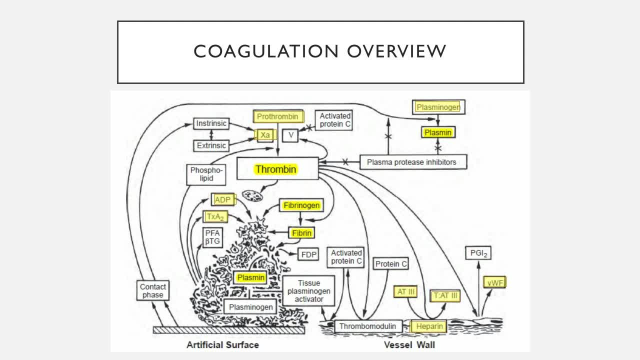 mechanisms that convert plasminogen into plasmin and that's actually reversing the process. On the right we see the von Willebrand factor that's necessary for platelets to adhere, that's being prevented from bonding by the vessel wall and natural surface, And we also see the 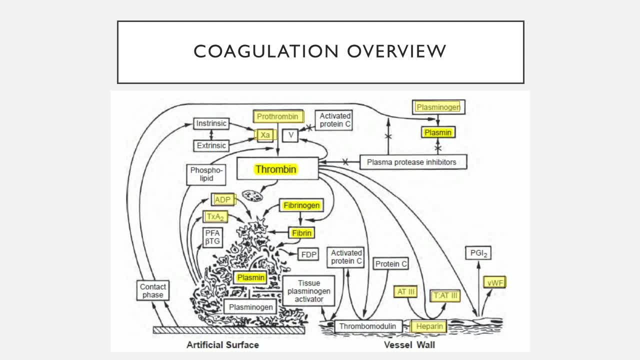 inhibitory mechanism of antithrobin-3, which binds to throbin to prevent it from activating platelets and helping them to adhere. We also see in that same part, with antithrobin-3 and the throbin-antithrobin-3 complex, the mention of heparin, a very common anticoagulant, And heparin. 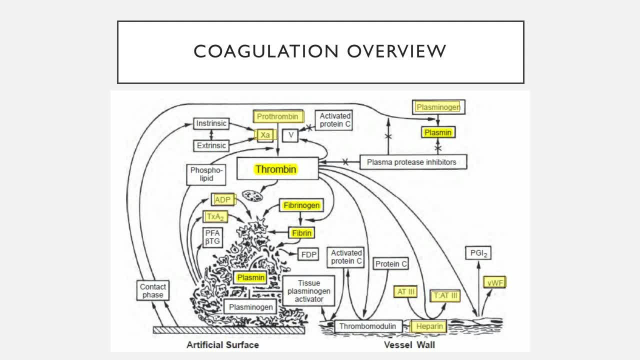 actually works by making antithrobin-3 orders of magnitude more effective in binding to throbin and preventing aggregation of platelets. So that's how heparin-3 works. We're going to close out the chapter by talking about bacterial infections. 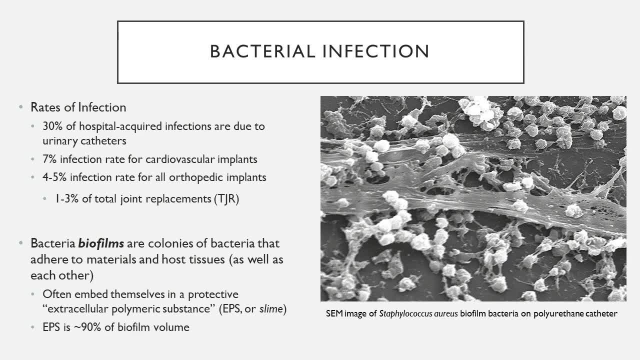 Now, ideally, biomaterials are always designed with the in mind that they're going to be implanted correctly and that bacterial infections which shouldn't be present after the sterilization of a process, after manufacture, shouldn't come up. But it's actually quite common in hospitals. 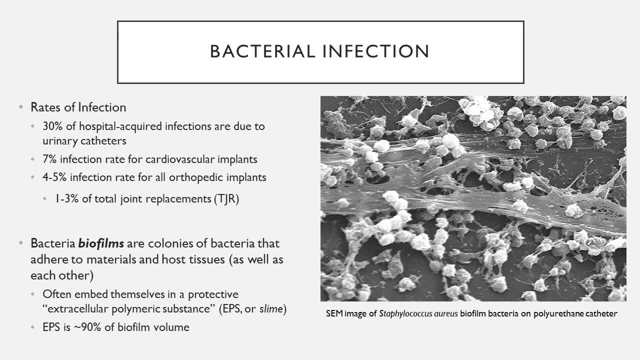 So to kind of give you an idea of the prevalence of these types of infections, I've gathered a few statistics here that kind of give you an idea of what the scope of this problem actually is. So 30% of all hospital-acquired infections are due to urinary catheters, a very common biomaterial, or 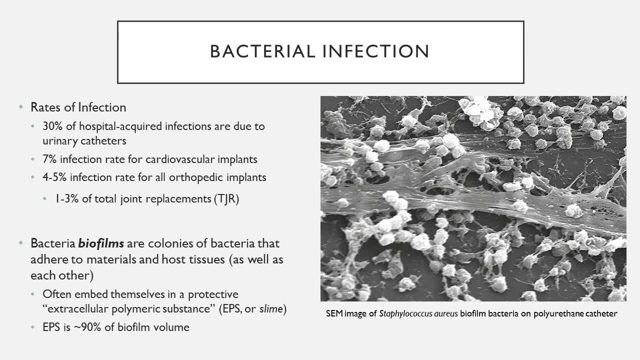 biomaterial device, I should say There's a 7% infection rate associated with cardiovascular implants and then a 4 to 5 infection rate for all orthopedic implants. Of these, 1 to 3% are associated with total joint replacements. So all of these are relatively huge infection rates And 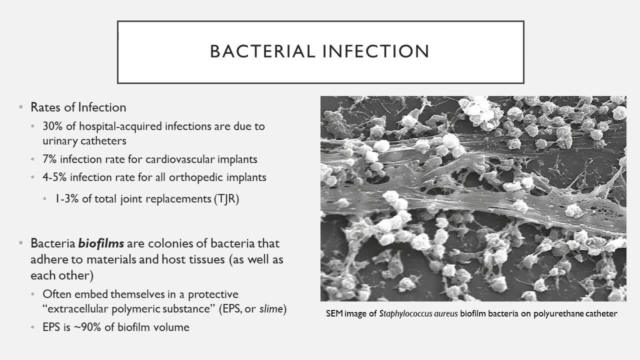 so whenever we're designing a biomaterial, we have to take that into account and figure out ways that could potentially be used, And so we're going to talk a little bit more about that in just a moment, But before we get into that, I want to talk a little bit more about some of the things that we can do to 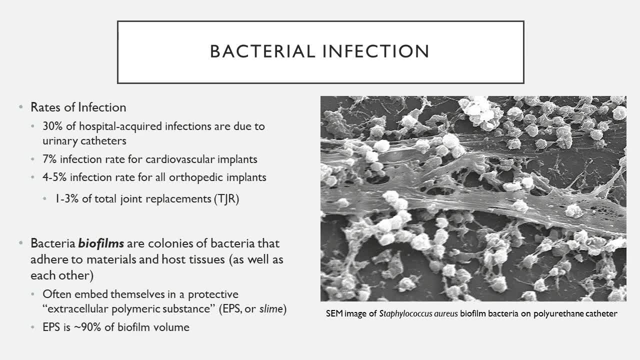 actually mitigate these problems In part. what makes bacteria so difficult to deal with is not singular bacterial cells that themselves can cause and spread infection. It's the resulting bacteria biofilms, which are colonies of bacteria that adhere to materials and host tissues, And 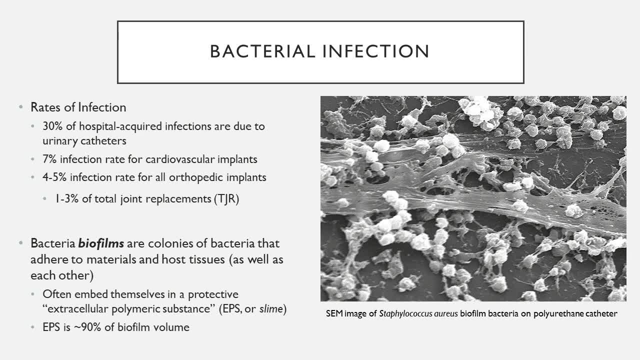 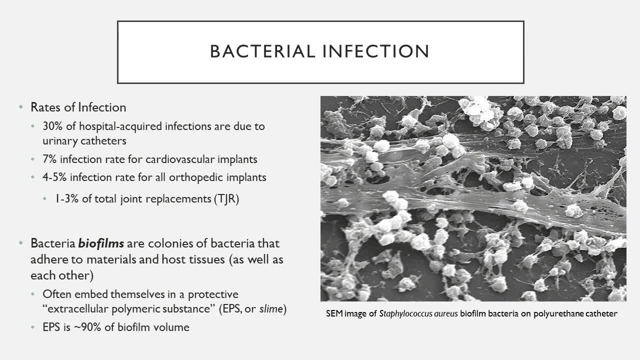 can actually see a picture of this. You can actually see a picture of this. You can actually see a picture of this using SEM images, like we have here on the slide on the right, and it's this biofilm that prevents a lot. 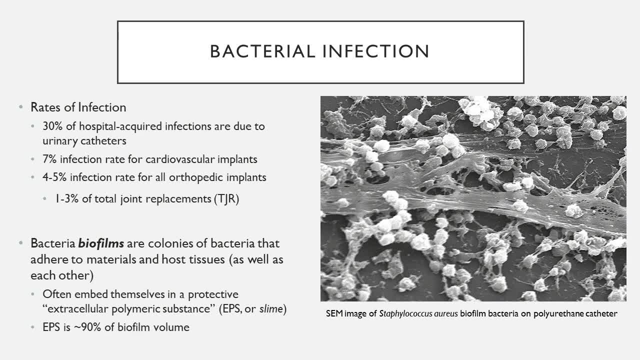 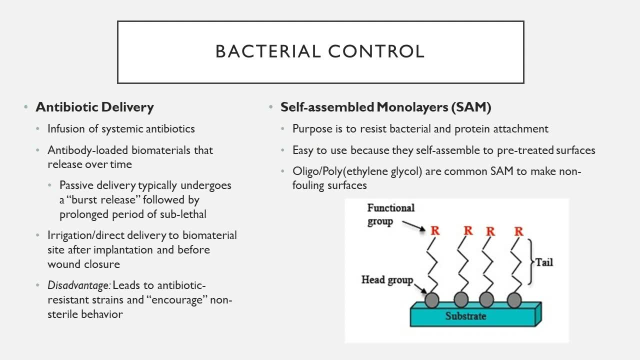 of current treatment methods from working in an efficace manner. There's a couple of ways the biomaterial scientists are using to control bacteria and incorporate some of these concepts into their biomaterials. The first has to deal with antibiotic delivery First. this can be: 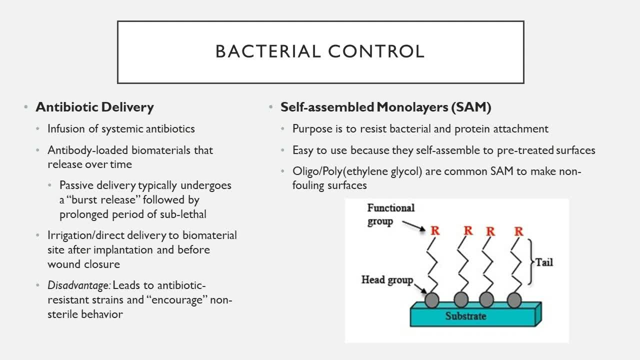 part of just standard operating procedures whenever putting in a biomaterial implant So you could just use. you could just take a sample. you could take a sample. you could take a sample. you use or rely on the infusion of systemic antibiotics. You can also load antibiotics. 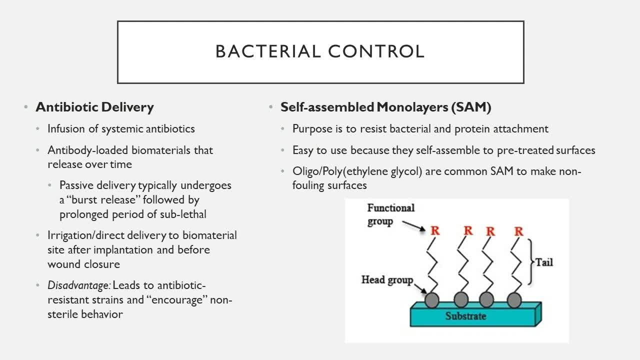 into biomaterials that release over time in a little bit more sophisticated manner. Usually, when done incorrectly, this kind of results in initial burst release that's followed by a prolonged series of sublethal release of the antibiotics. So scientists need to make sure that 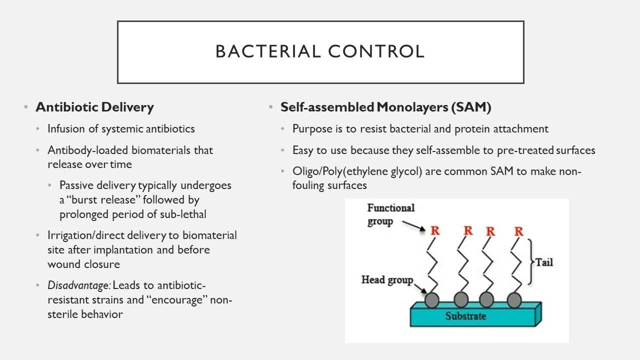 they can tailor and maybe do like a zero order release profile that releases antibiotics and doesn't waste all on initial burst but has a prolonged period of lethal release. Surgeons can also implement a direct irrigation or delivery of antibiotics to the biomaterial implant site, either after implantation or before wound closure. Now, in general, the big disadvantage with all these. 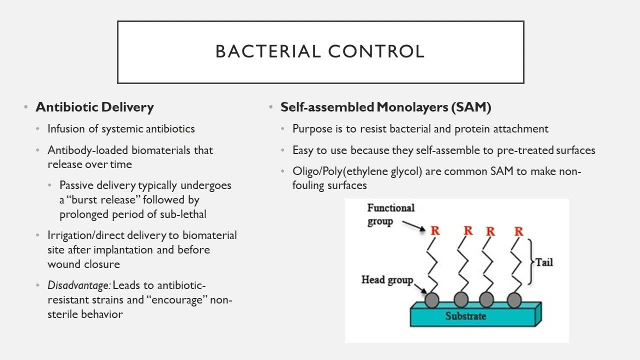 methods is that they lead to antibiotic resistant strains of pathogens and they also, to some what degree, encourage non-sterile behavior. If a surgeon or a scientist can rely on the bacteria working, then we have to worry less about keeping clean methods if we know. 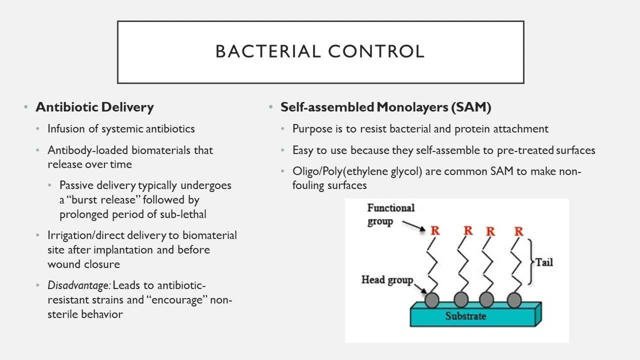 we can rely on this. There's also more passive ways of fighting bacteria that don't involve trying to kill the bacteria directly. One of those is the use of self-assembled monolayers that are on the biomaterial surface that resist bacterial and protein attachment. 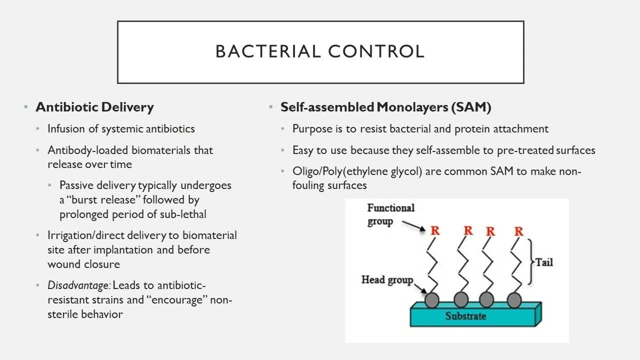 Now what's nice about these self-assembled monolayers is just that implied in the name: They self-assemble themselves, so they're actually easy to use. So we can just use some basic chemistry and apply some really passive, non-reactive functional groups of surfaces that align themselves in just a thermodynamically and chemically favorable way. 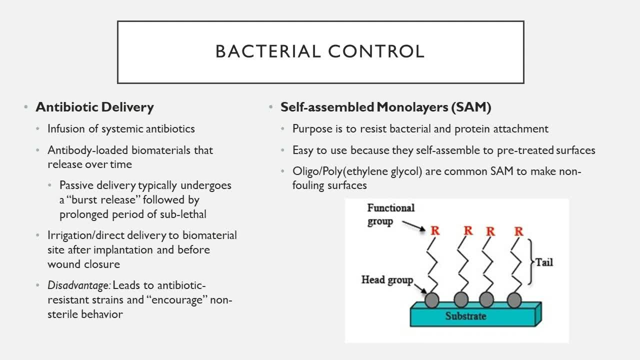 Very common molecule used for this is polyethylene glycol. because it's non-reactive, PEG is used in a lot of FDA approved devices. The FDA loves it itself and it's non-fouling, so it's a very common way of hiding things and preventing the adherence of proteins that either the immune system would. 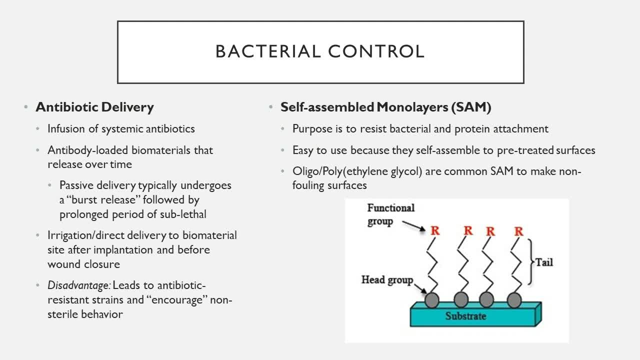 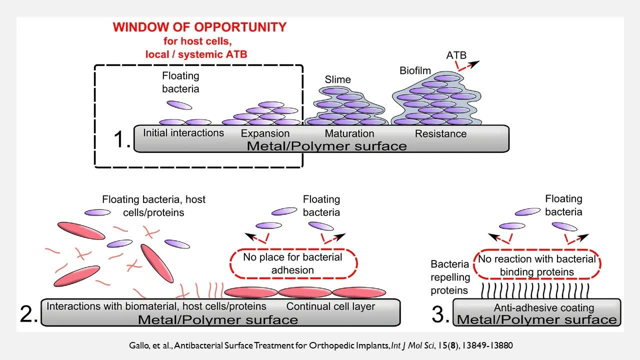 recognize or bacteria themselves would directly recognize. A nice little overview of the biofilm process and the adhesion strategies can be presented in this diagram here below, And something I want to point out here is something known as the window of opportunity, where a small amount of bacteria 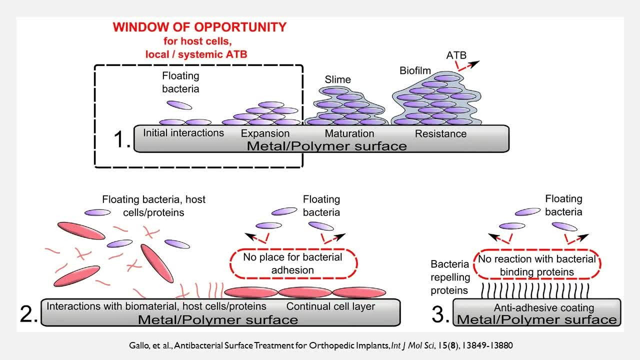 has to first build up into the initial formation of this colony before it starts secreting the slime material that EPS that eventually makes a thick colony with this heavy biofilm surrounding it that makes it so. So the first step is to build up a new cell that is resistant to antibiotics. So scientists form most of their 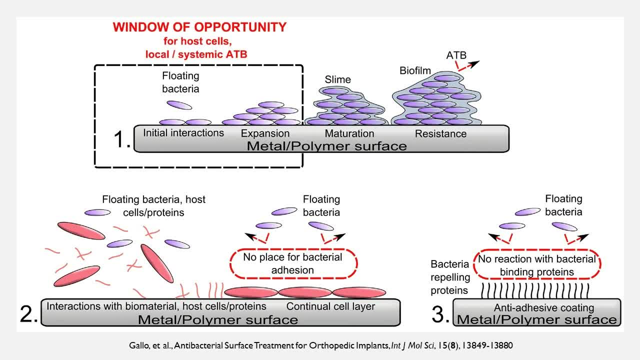 strategies in preventing the formation within this window of opportunity, knowing that it's a lot more difficult once the slime and EPS is developed. One way to promote this is actually to encourage our own host cells to adhere to biomaterials and rely on non-inflammatory cell reactions to our biomaterials. 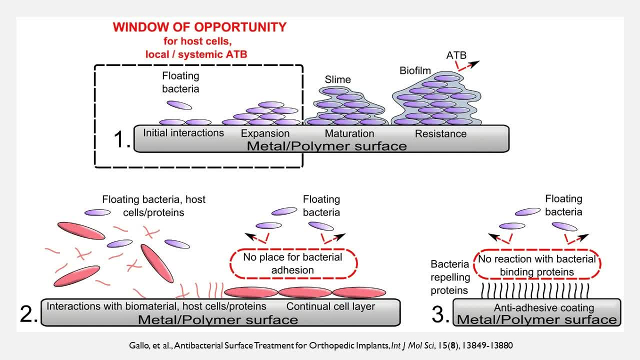 so that they themselves kind of form a coating, a nice safe coating on the biomaterial that prevents host cells from adhering to it. Then the last one is- just like we discussed on the previous slide, some sort of non-adhesive coating, like with the self-assembled monolayers that prevent both host cells and bacteria. 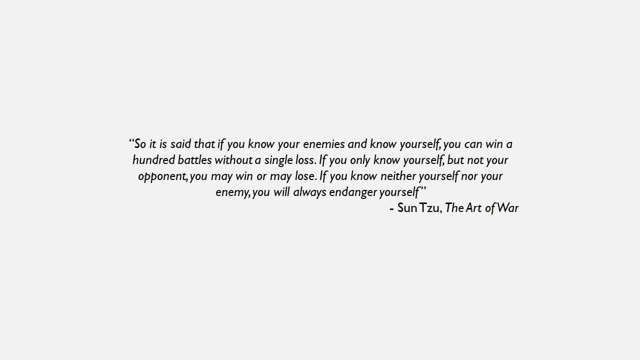 from attaching to it. So that concludes this chapter on the background of cells, both foreign and host cells that could potentially react against biomaterials. So I think it's appropriate to end with this. know your enemy-like quote from Sun Tzu. In the later chapters we'll discuss the 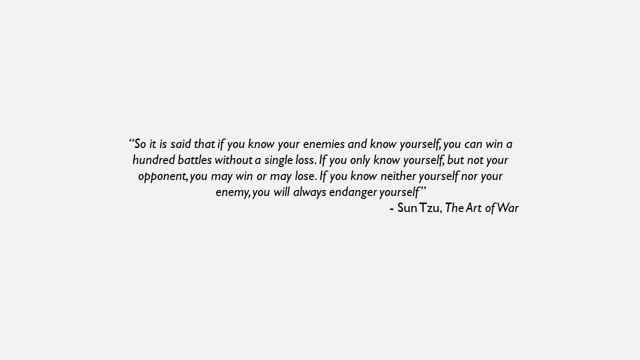 ways that scientists evaluate biomaterials now, knowing these background concepts, So we'll take it from there. Thanks for listening. 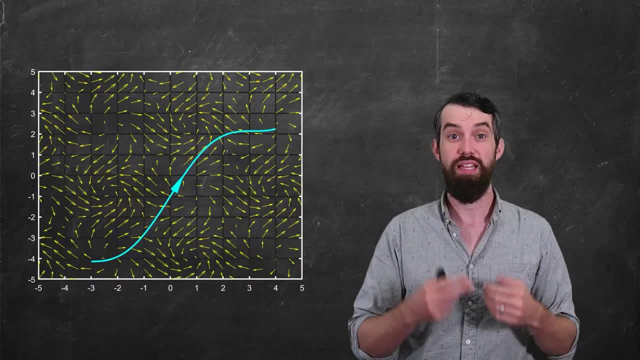 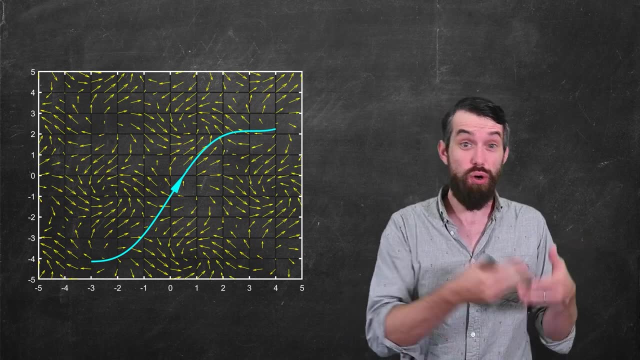 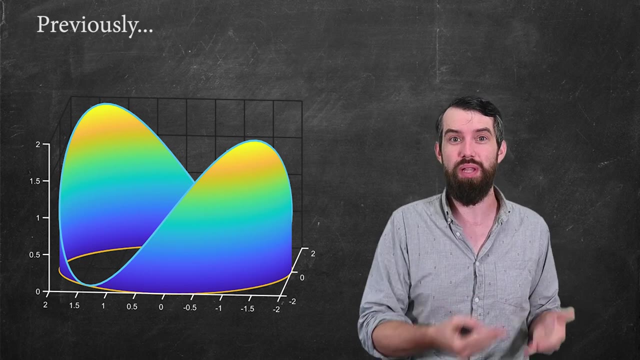 In this video we're going to talk about the line integral of a vector field. We previously have seen line integrals earlier on in my playlist on vector calculus- The link to that playlist is down in the description- And when we previously talked about line integrals, we would have some path. 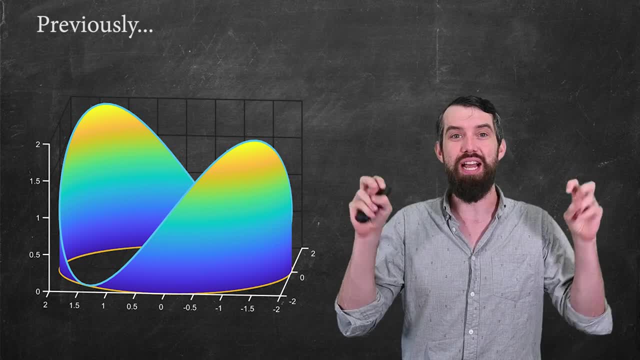 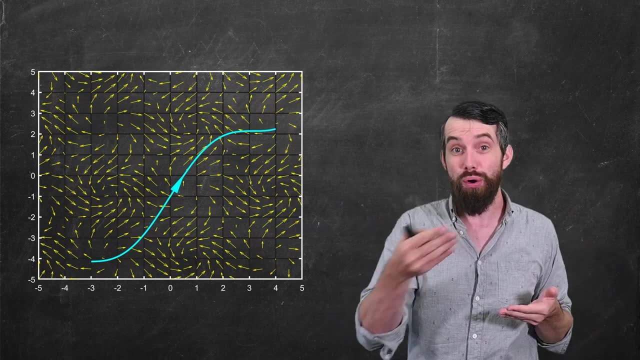 and then we had some function that gave a sort of height above every point along that curve. But now we're imagining a scenario like this where we've got some vector field and we've got a curve that is moving through the vector field And if you look at this vector field- sometimes the arrows- 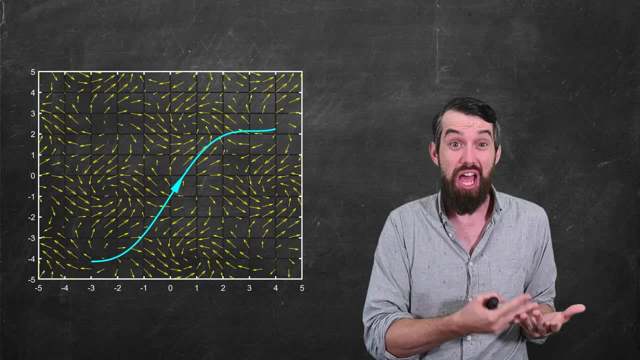 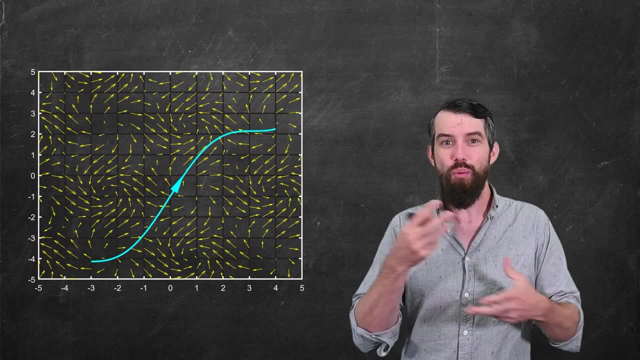 of the vector field appear to be almost tangent to the curve. Sometimes they're pointing completely away from the curve in all sorts of directions. What we want to try and measure here is some way of capturing the degree to which the vector field goes along with the path of the curve, and that 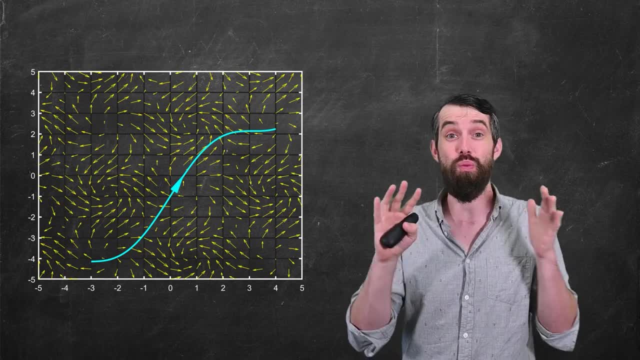 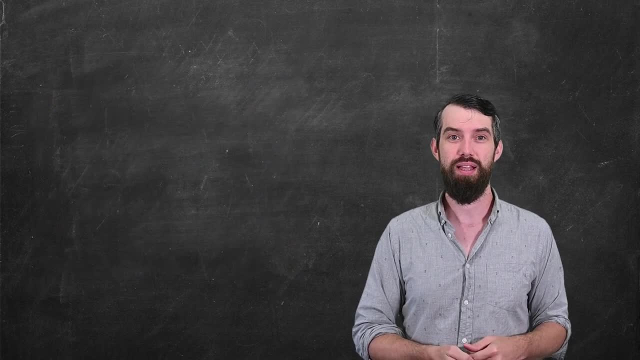 the tangent of the curve and the vector field are aligned. So what does that mean? Well, let's start with a more concrete example from physics: The concept of work. Indeed, you might recall that work was defined to be a force times a distance.